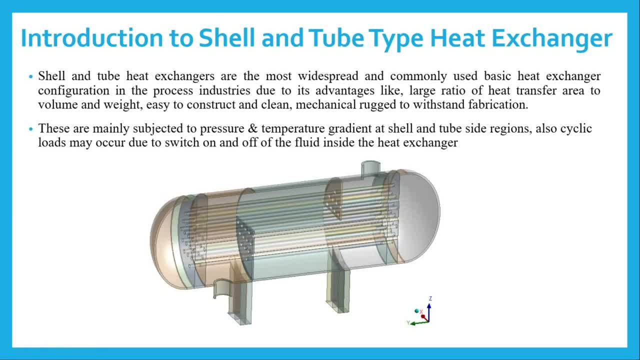 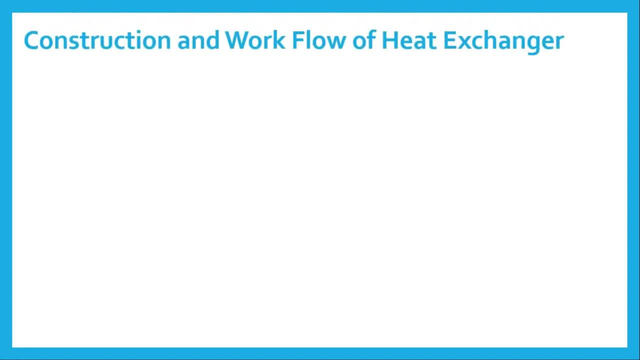 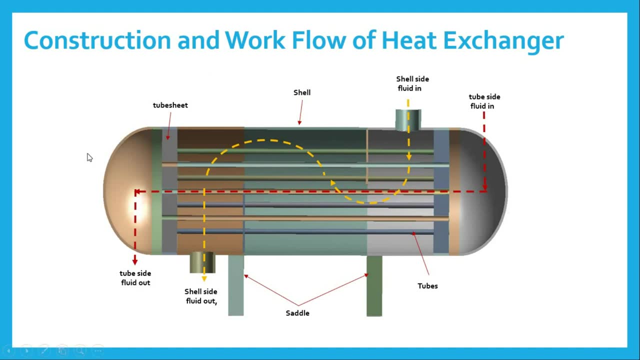 of shell and tube type heat exchangers. we will see the more construction of this in next slide so that we will get some idea. so if you see this schematic, represent the shell and tube type heat exchanger, this outer portion is nothing but your shell and these are the heads right. and if you see 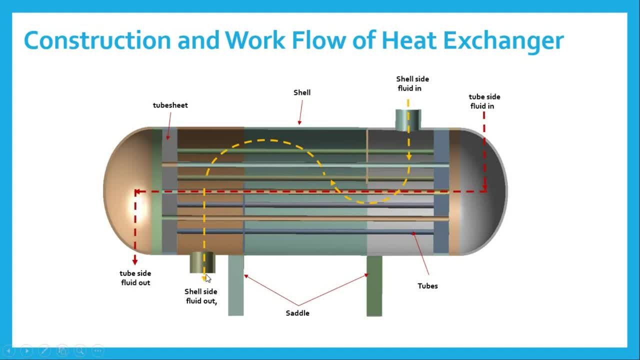 these are the tubes and this is tube sheet and these are the nozzles, and the base is nothing but your saddle. so these are the major components of any heat exchangers, like tube sheets, your shell and the nozzles from where the fluid will come into picture. so when we talk about shell and 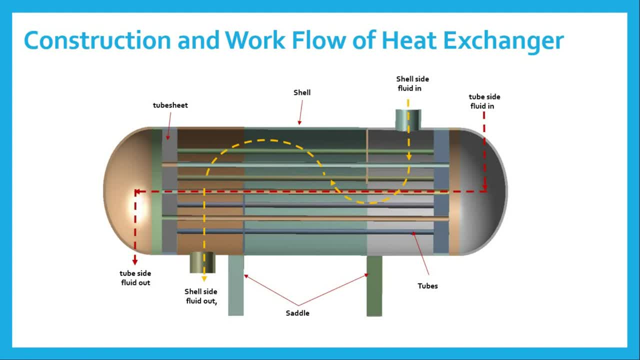 and tube type connection. there are two things will come into picture: tube side as well as shell side. the tube side is nothing but the side in which the tube side flow will going to flow. suppose there will be, in actual there will. one more lonzer will going to be here. 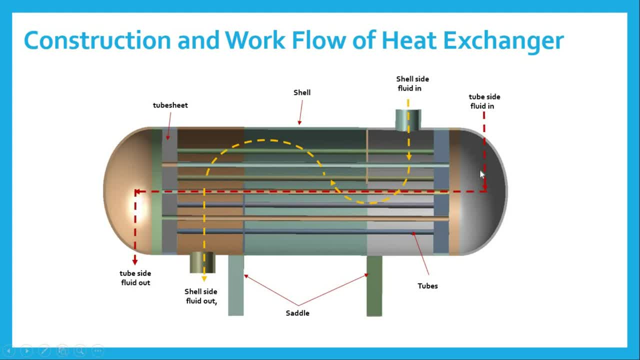 and from that nozzle the fluid will come into this region and it will go inside the tubes and then it will come out from this. so this region where the fluid will come into picture, this region is nothing but. your tube side region and shell side region is nothing but. 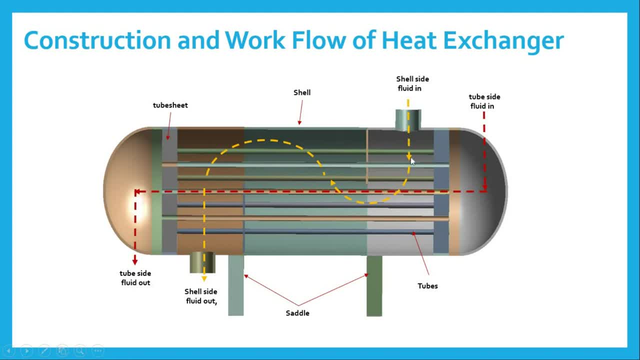 the fluid which will moving over the tubes. you can see from this like this: here you can see these are the baffles which allow to make maximum heat transfer area ok. so there might be different duty cycle, one of the duty cycle when the equipment will going to start and 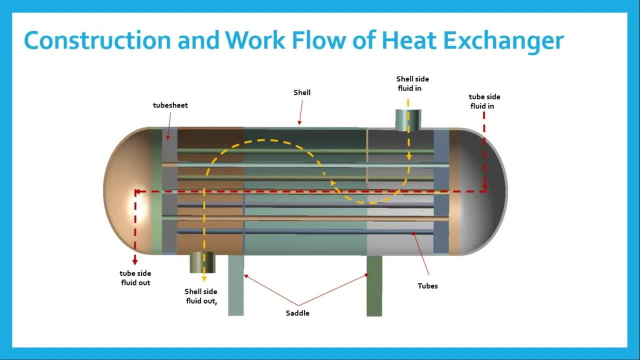 when equipment going to shutdown. So in this kind of shell and tube type heat exchangers, these are basically subjected to thermal as well as pressure loads- may have possibility to cause the thermal fatigue because it is subjected to different duty cycles which are having at high temperature reasons, as 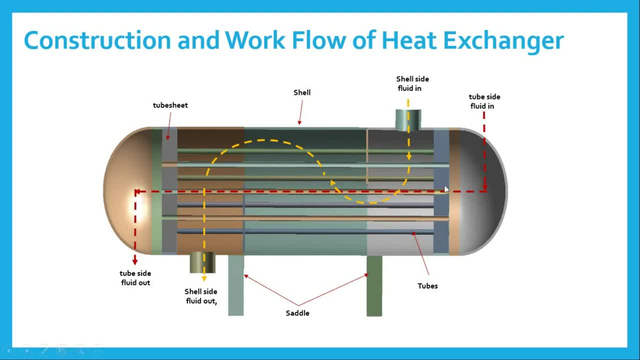 well as some structural failure which will going to come, and most of the stresses are developed at this tube to tube sheet junction, this junction, as well as tube to tube sheet and tube to shell junction, because here you will find the more temperature gradient. also some of the failures at the saddle support, because here we will going to fix ok. 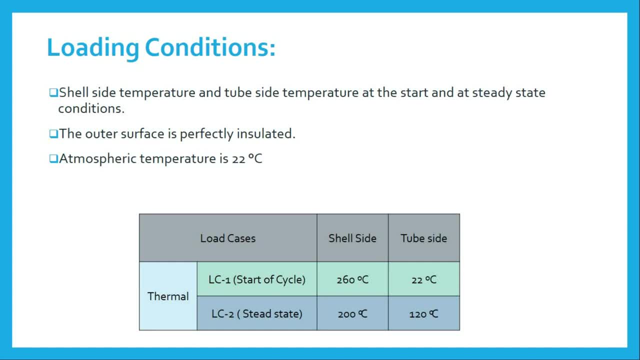 So these are the loading conditions in this. so if you see first the shell side and tube side temperature at the start and at the steady state conditions so they wanted here, we need to simulate the temperature we are at the start, At the start of the heat exchanger, as well as once your after an hour, you will get some. 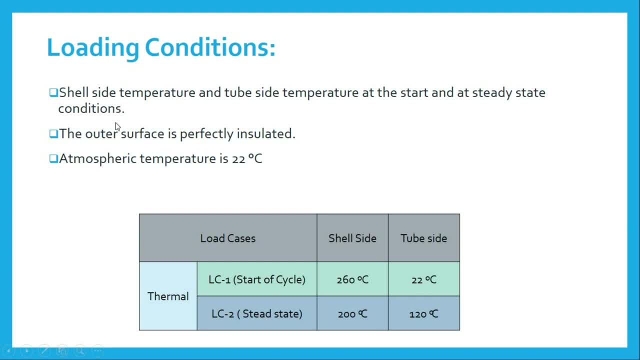 steady state condition. so that condition also we need to simulate. then the condition like outer surface is perfectly insulated and also having atmospheric temperature of 22. so this tabular section represent the first load case. that is your start of the cycle and the shell side will be 260 and tube side will be 22 and here, like once, steady state is available. 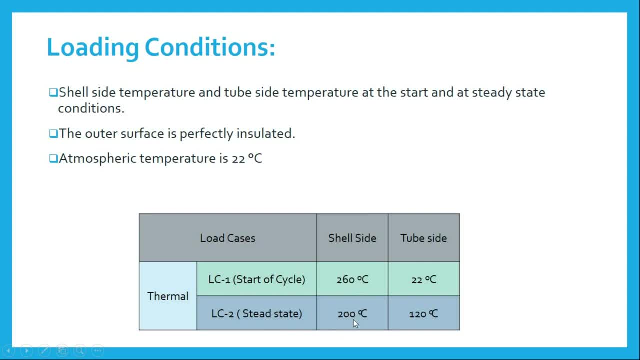 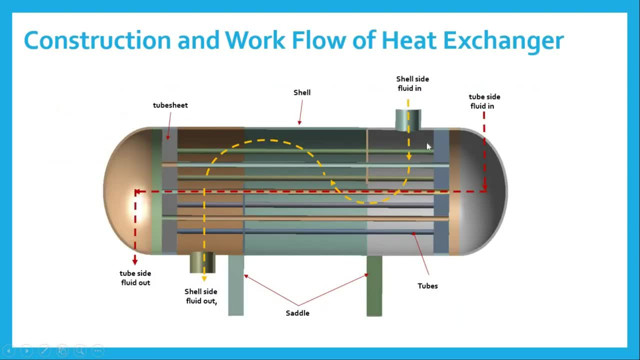 this 260.. Ok, So this 260 will going to reduce up to 200 and this 22 degree centigrade will going to increase up to 120 degree centigrade. so if you see here, so here at the start of the cycle. 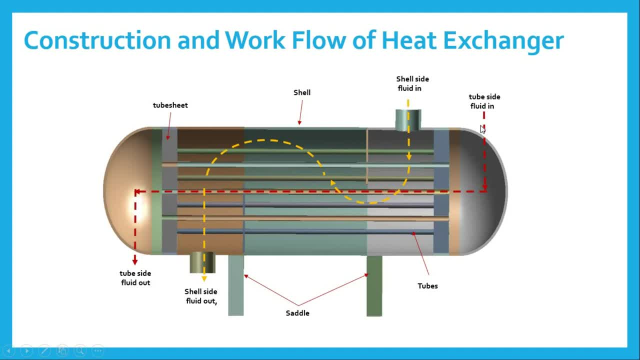 here it is like 260 degree centigrade and at the start of cycle it will be like 22 degree centigrade. so once equipment will start running, after an hour you will find this temperature of shell side which is at 260. it will going to reduce up to 200.. 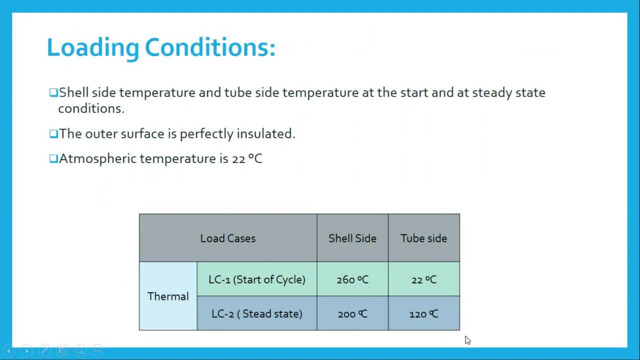 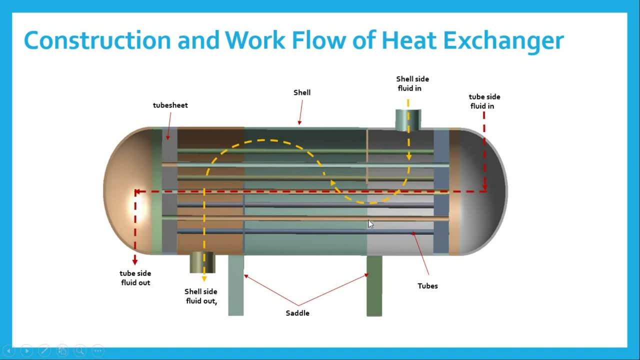 This will going to increase up to 120 degree centigrade. so this is due to the heat transfer will going to happen between shell side and tube side. Ok, then we will move towards our actual simulation part in ANSYS. there we will try to simulate. 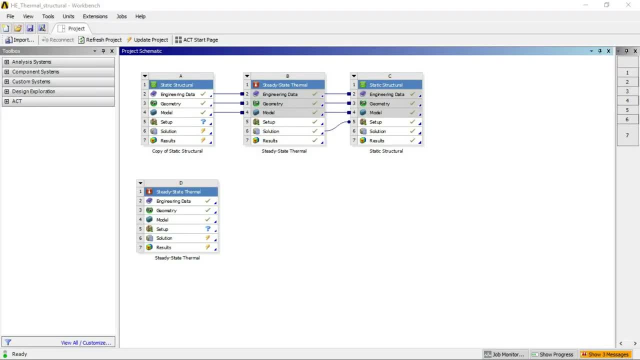 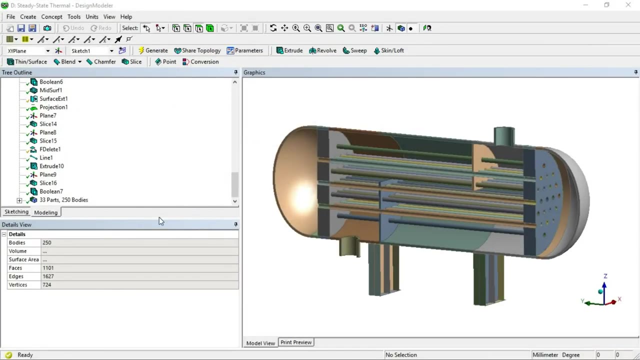 this conditions. so now we will move towards our actual ANSYS part. before proceeding to this, you just cross check with the unit first and this drag and drop your steady state thermal module. Ok, once it is open, you just go to geometry editor and you can read the geometry. 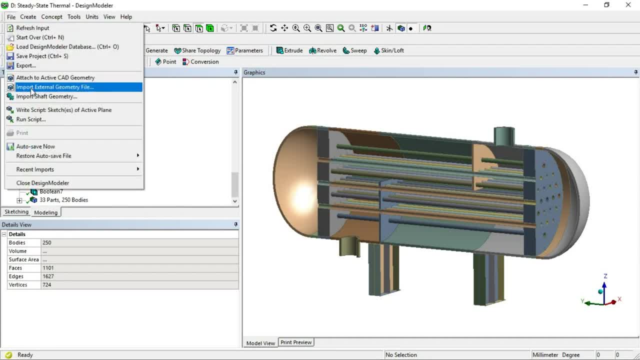 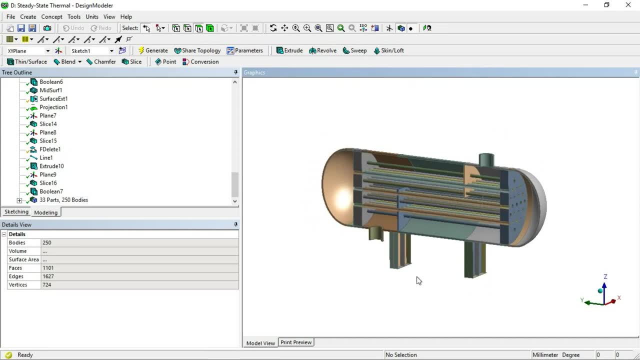 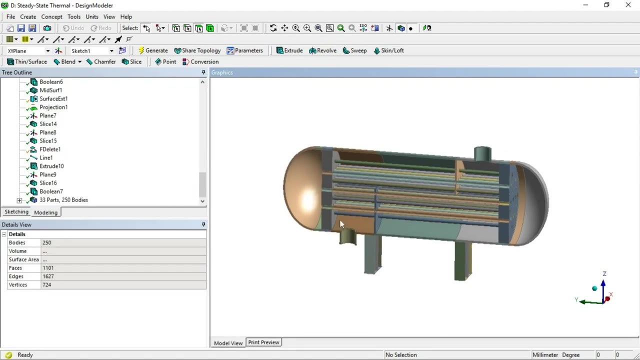 from your local directory, like from file, import external geometry file and then give the path of that respective geometry. okay, so this is the model which I actually created in design modeler itself. if you also want to create you, just refer my another video which explains about how to create vertical. 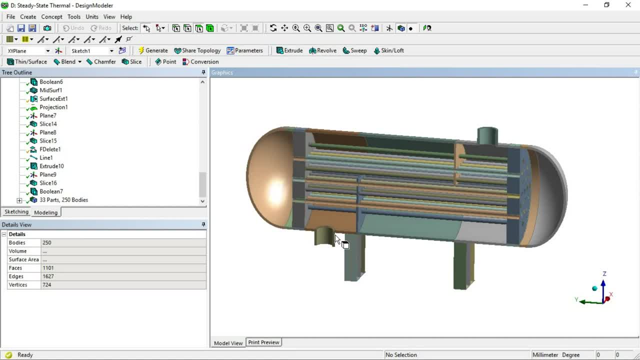 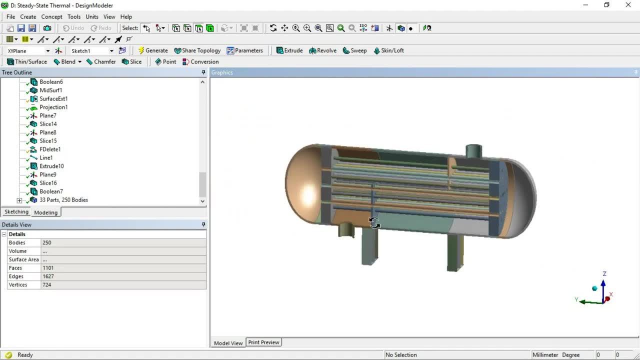 pressure vessel using ANSYS design modeler. so there, you will get some idea how to create this much when this kind of geometry will be there. okay, so this geometry, as we discussed earlier, it may consist of your head, this is what your shell, this is your nozzle, and which are supported by using these saddles. okay, 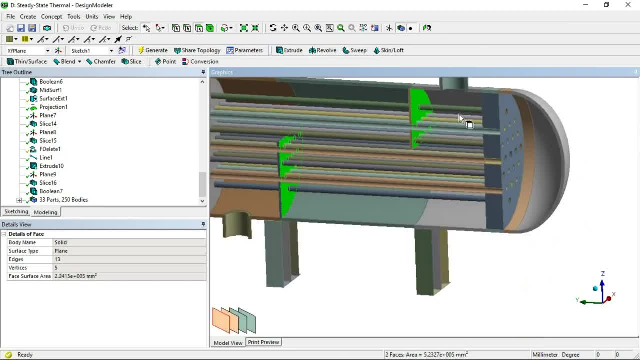 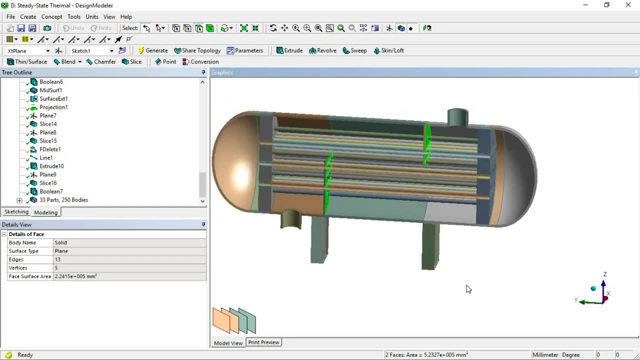 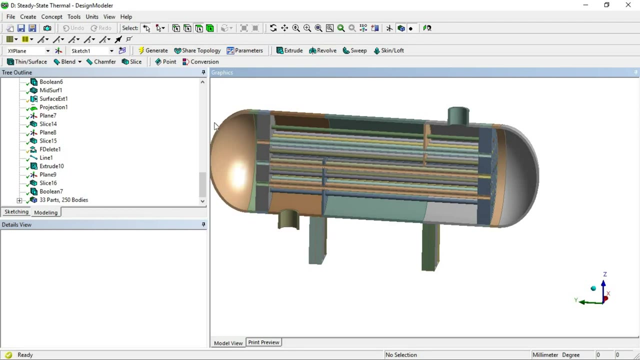 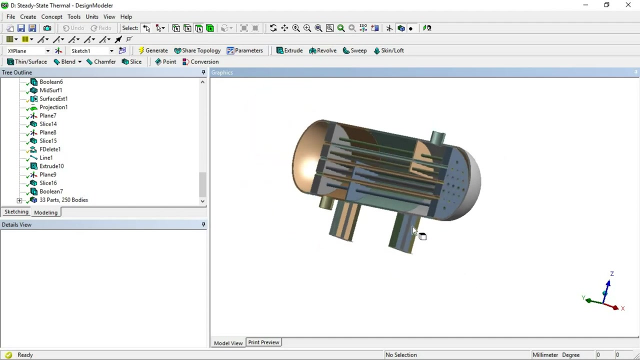 and these are the baffles and these are the your tubes from which your fluid will going to flow. okay, and as we discuss regarding shell side and tube side, the shell side fluid will discuss that in mechanical window here like this: is what your complete solid model- and I had created this saddle using shell model just to reduce the 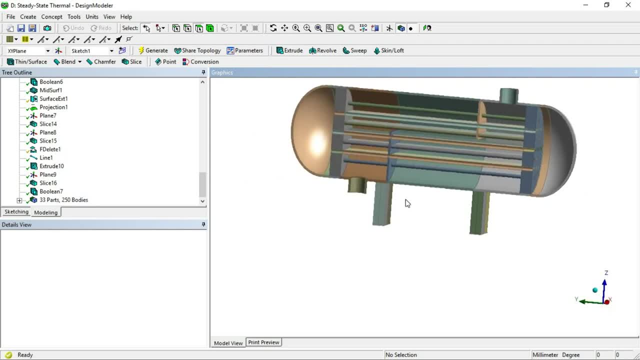 mesh count. okay, you can do also at your handle, even here also. it is possible to extract the shell for complete vessel also, but there you will not able to find the gradient, so that's why it is mandatory. you can extract the shell for complete vessel also, but there you will not able to find the gradient, so that's why it is mandatory you can. 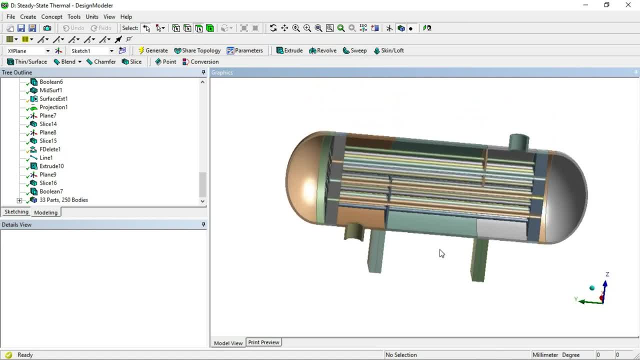 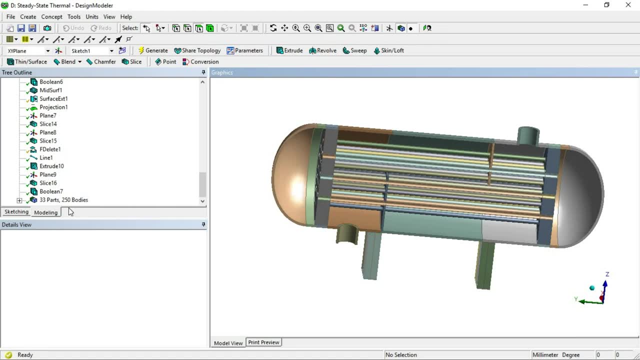 go with the solid elements when you will going to do the thermal solutions and you want to see the temperature gradient across the thicknesses. okay, once it is done, you just create a different parts for your solid bodies and, as these are like shell bodies and different parts, are your solid bodies shell and different. 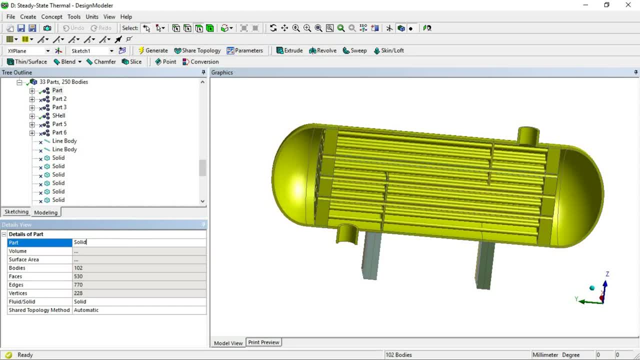 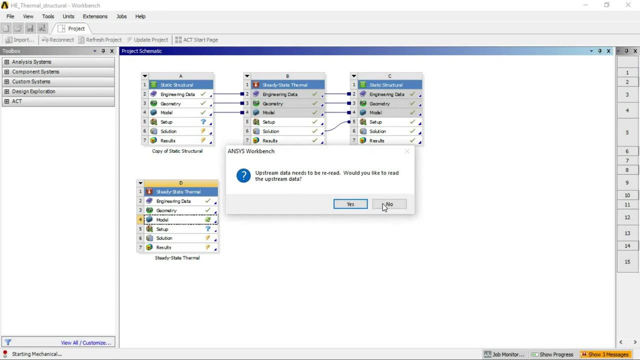 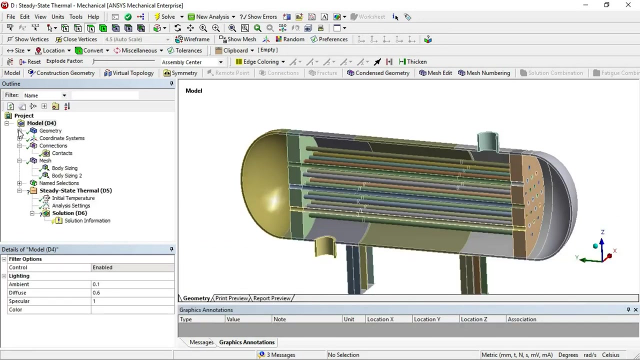 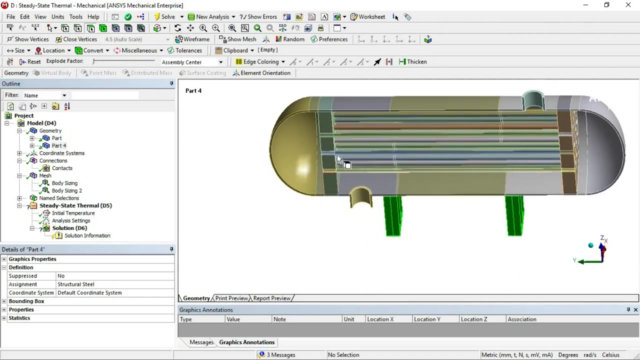 parts for your solid. okay, Now we will move towards a. once it is done, your geometric clean up and all the settings, you just quickly move towards our, your mechanical window. so here you will find that geometric definitions, and there, here also, you can find this is sheild part. okay, now working to the first, we need to cross check with the connections. so here this is now. the thing is that initially, 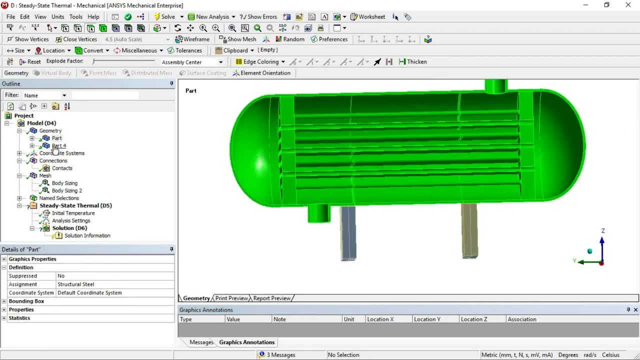 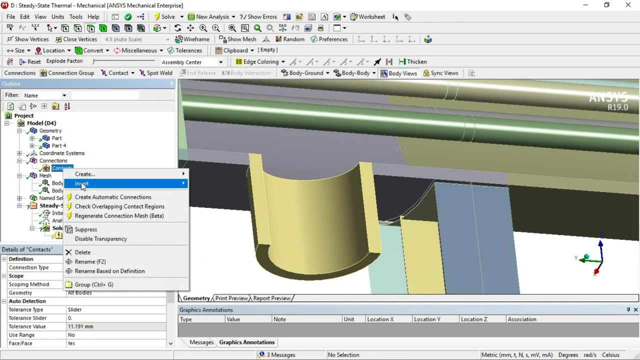 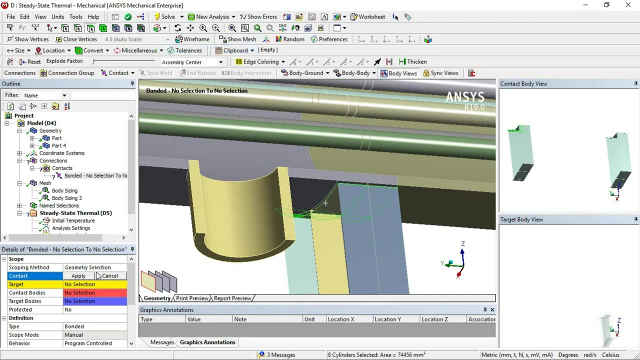 this is the single part, so there is no need to define any connection. but here it is different part, so you can define a connection between saddle and shell. okay, so here right click, insert manual contact region, select these two different surfaces. here no need to worry about shell and tube side, because that will not going to. 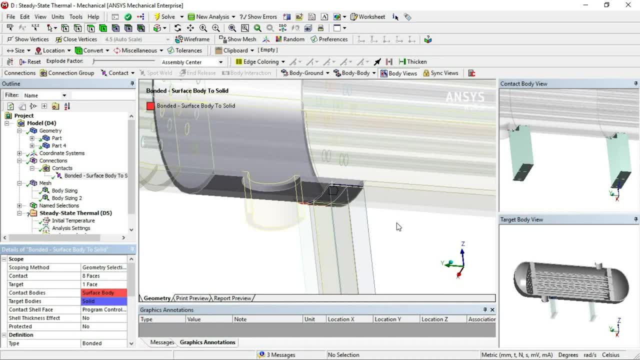 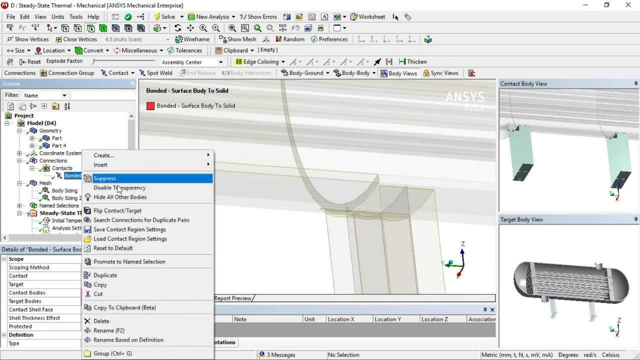 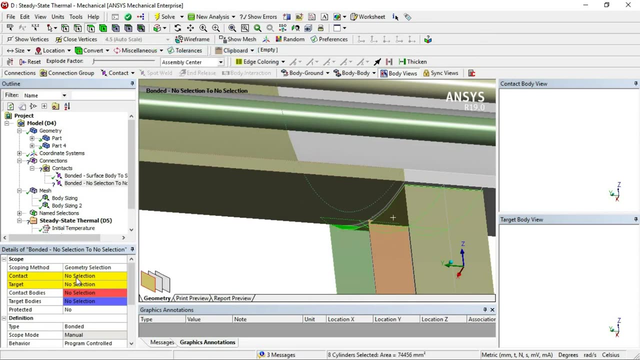 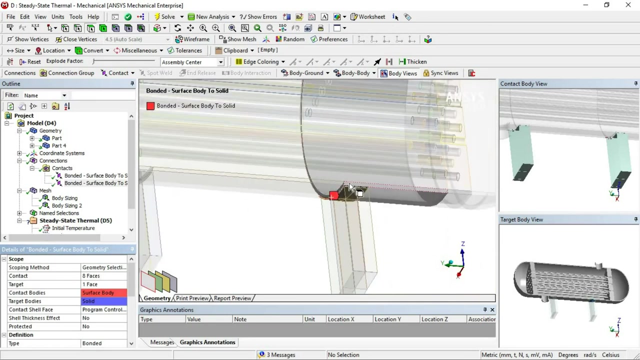 create much more impact. and this is not your non-linear simulation. this is straightly linear and which is very much straight forward. so no need to worry about your shell side- sorry. contact and target definition in contact. okay, once your contact is done, you just define your meshing, create your mesh. here, actually, i did some. 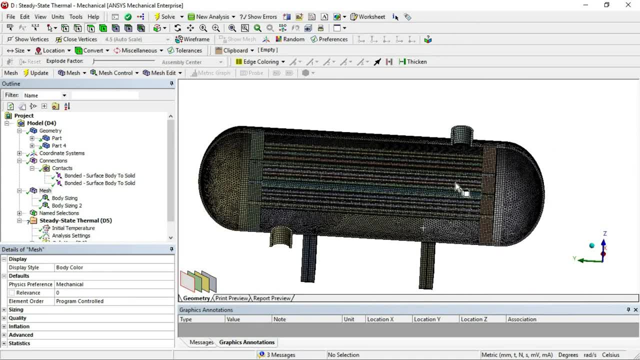 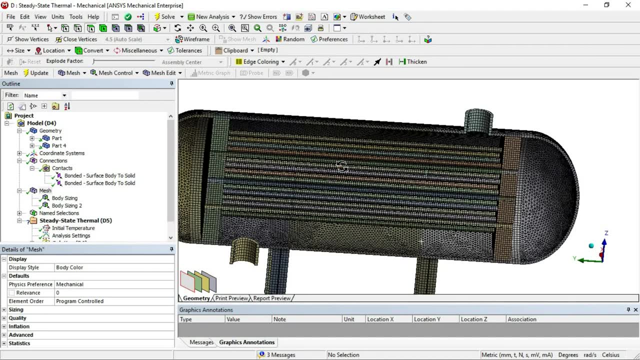 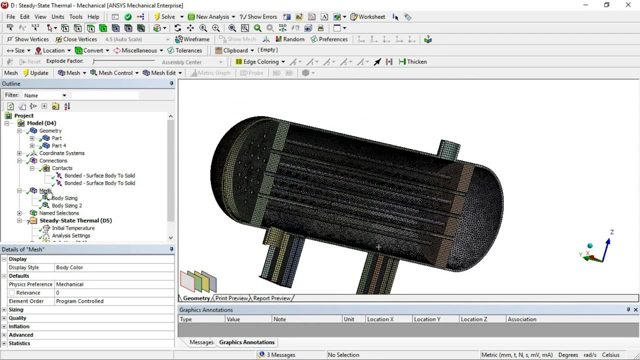 coarse mesh. but it's not necessary, because, just to get the faster solutions at your end you just go through at least 3 elements across the thickness and also, if it is possible, you just keep 2 elements across these tubes right and once your meshing is done, you can move towards your actual loading condition. 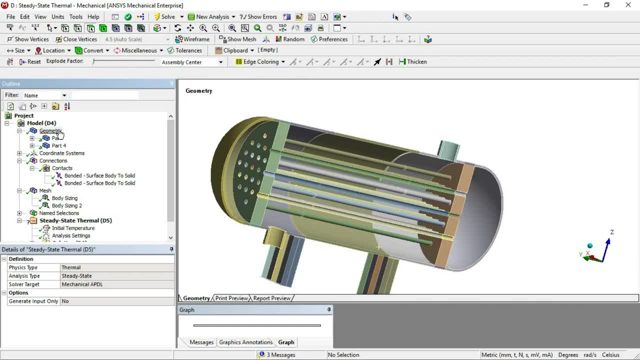 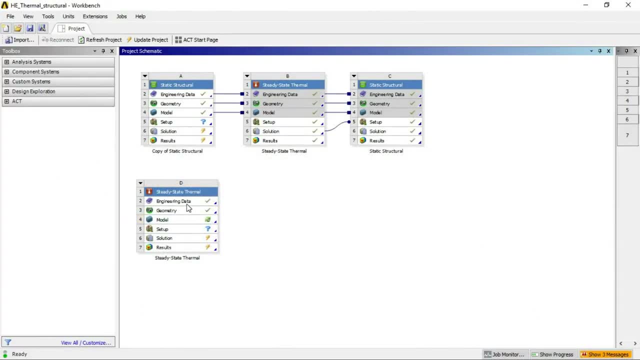 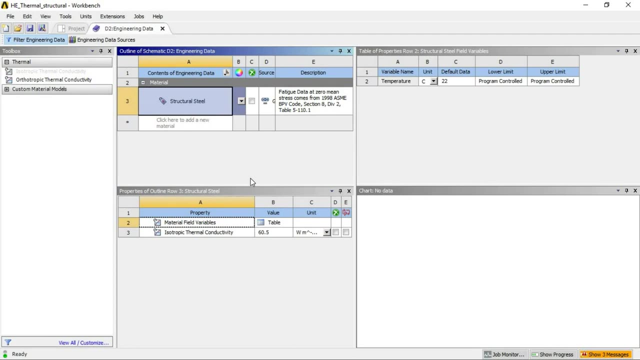 but before loading condition, you just make sure that your material definition- right now it is by default, structural steel. so what i will do, i will create a material definition. you just go to engineering data. so when you do, you are doing any thermal simulation. so there are like important thing that you need to define the thermal conductivity which is. 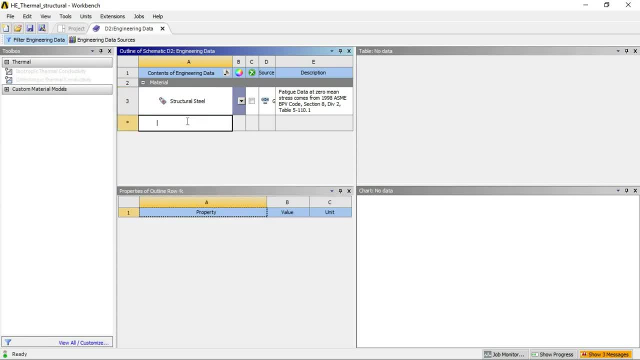 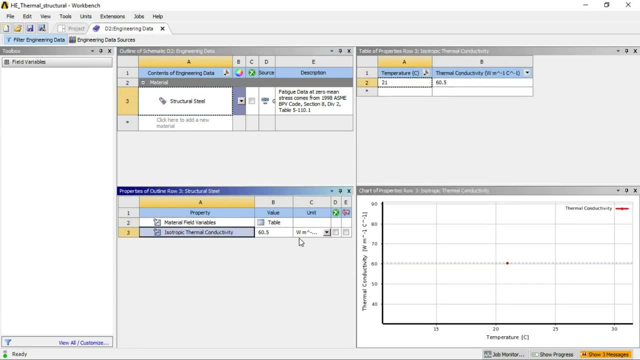 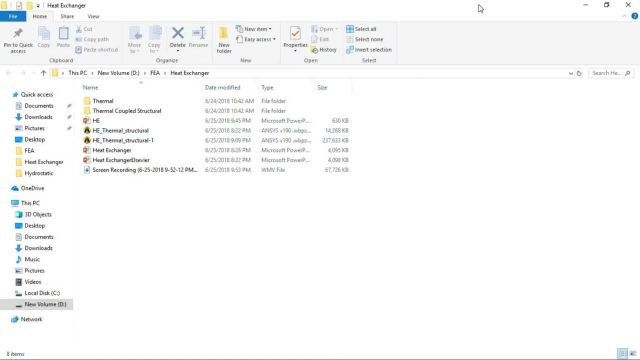 very much important. you can see here, this is a by default your structural steel material, and here you will find the thermal conductivity which is like 60.5 watt per meter per second. kelvin max per meter degree centigrade. you can see right, so that is a very much important. 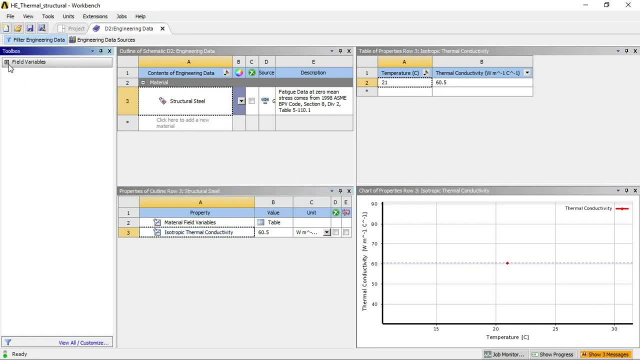 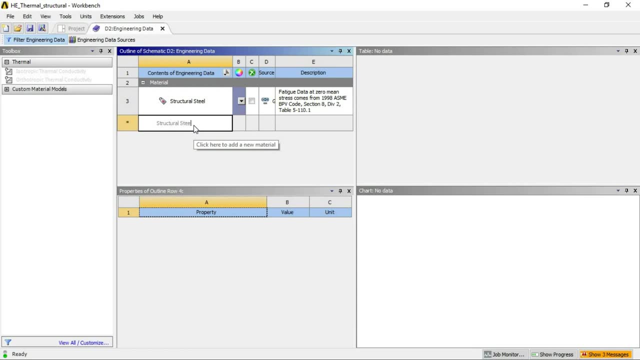 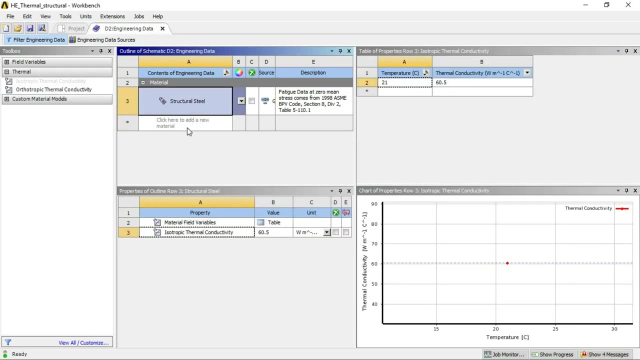 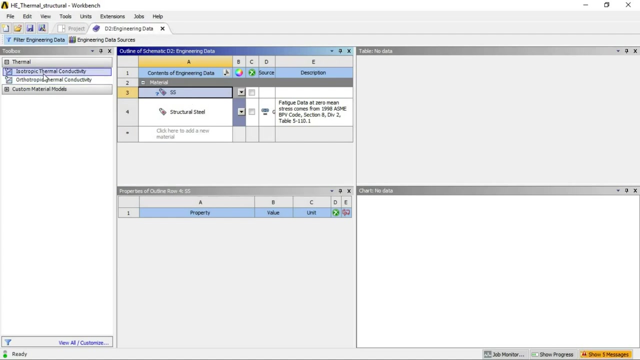 when you will going to do the thermal simulation. so how you can define that i will tell you. you just go here, put structural steel right. it is already there. that's why it is not coming. so control c, control v. i will write ss right and here you can see, here, thermal definition, so you can define your like 60.2 or water. 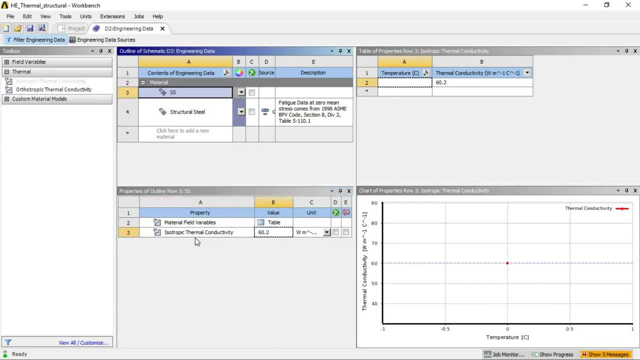 it may be like that you can define your structural steel. there is one. when you will couple this structure- thermal simulation- with structural, then you will find there more definition of material. so there we need to define your young's modulus, then we need to define poisons ratio. 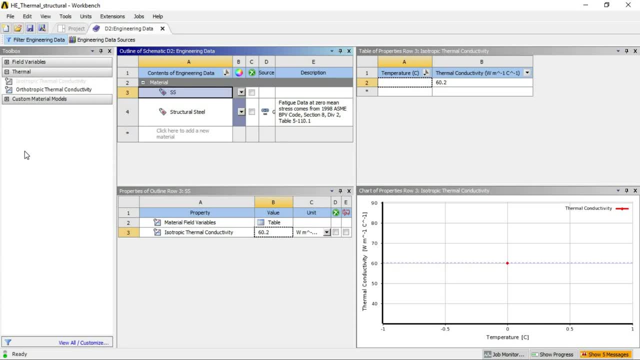 and then we need to define the thermal expansion coefficient and also we need to define the heat. so if suppose you are doing transient thermal, so in that case we also need to define the specific heat. okay, so if you have different material details, like different thermal conductivity in different direction, in case of orthopedic, orthotropic, you can define from this also. 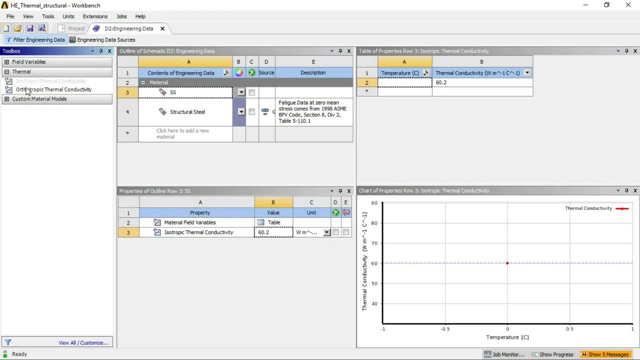 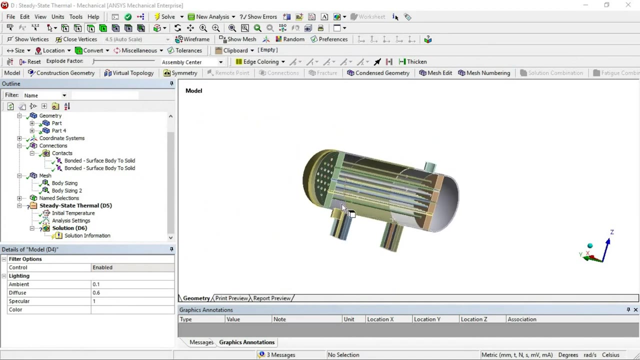 but i had seen, like most of the customer, or you can say, the most of the equipments lie under the isotropic thermal conductivity. so this is what your assumptions. okay, so once your material is defined, you just quickly move towards your mechanical window. i will not update this because it will take time. so once it is done, the very first thing that 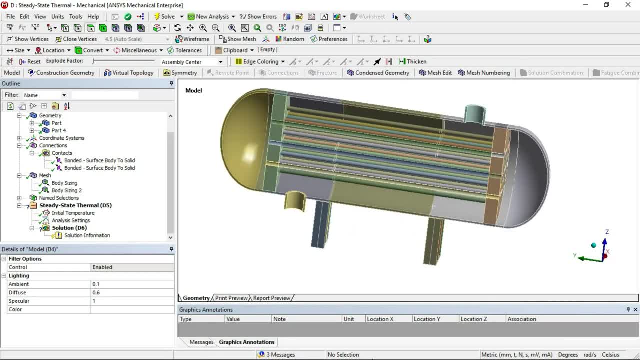 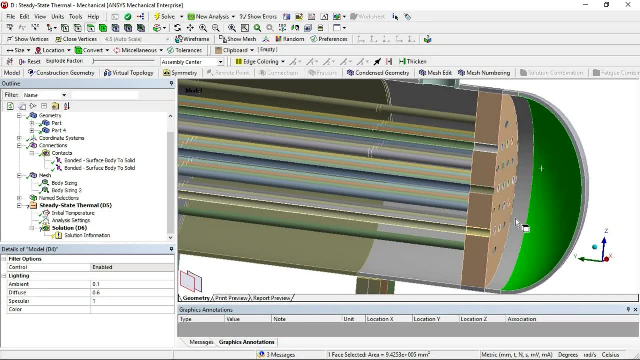 you just create the name selection for your shell side and tube side because, if you see, our temperature definitions are like that. so i will create the name selection first. i will select the what is the tube side region so that you will also come to know. i will 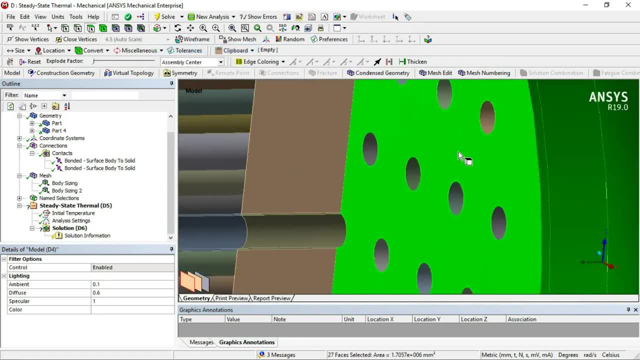 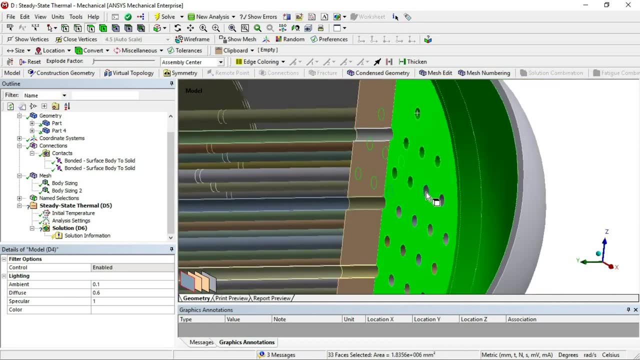 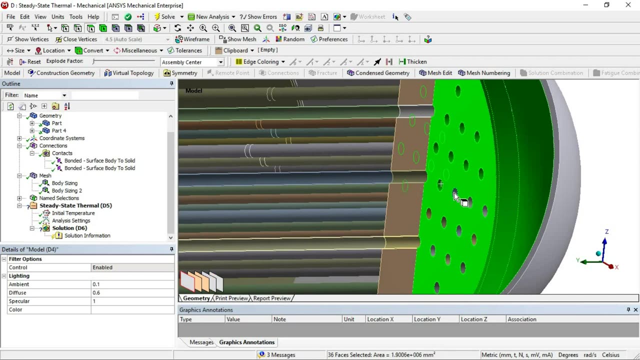 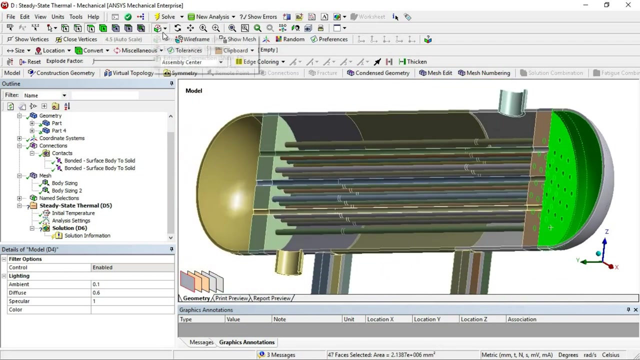 select all these parts. i will keep extend to limit, okay, and i will select all the inside tubes. reason: because the fluid which will come in tube side will move under this tubes and will flow from this side to that side. okay, once it is done, you just further do extend to limit so you will find all the internal. 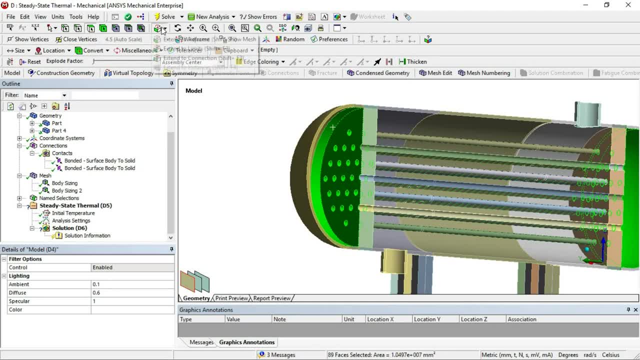 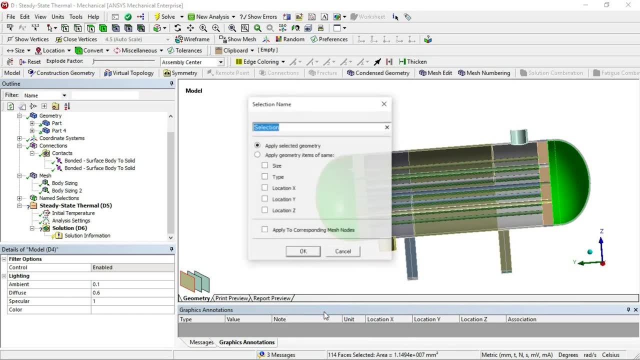 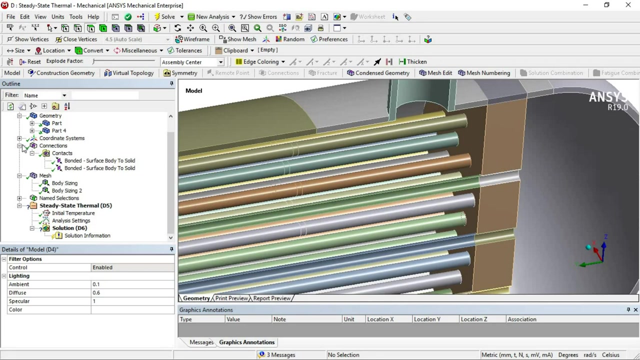 surfaces are selected further. do extend to limit. okay. so this is my tube side reason. insert. create name selection. put here tube side reason: okay. similarly, you can create a shell side reason, so shell side will be above the tubes. I think here we had missed something. I will suppress. 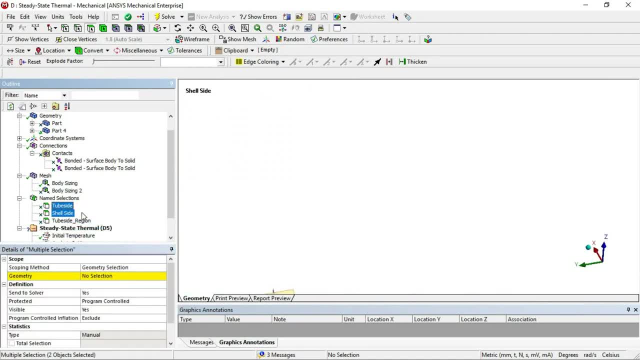 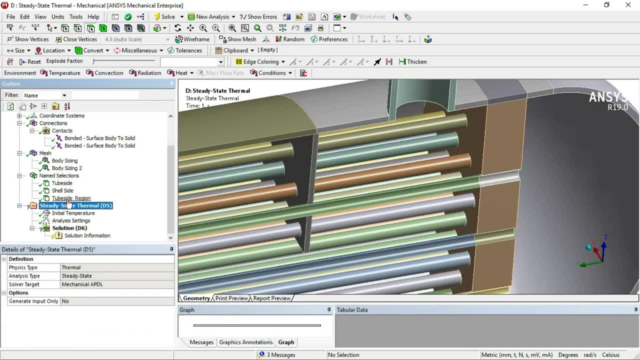 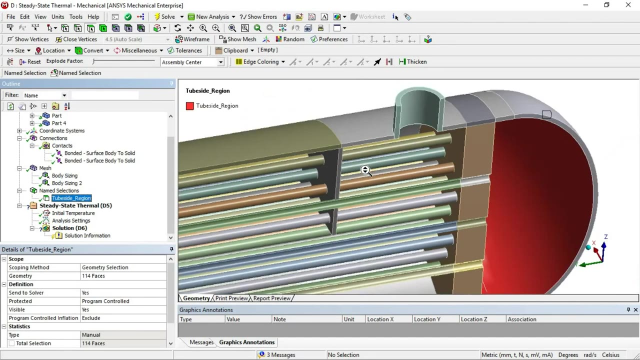 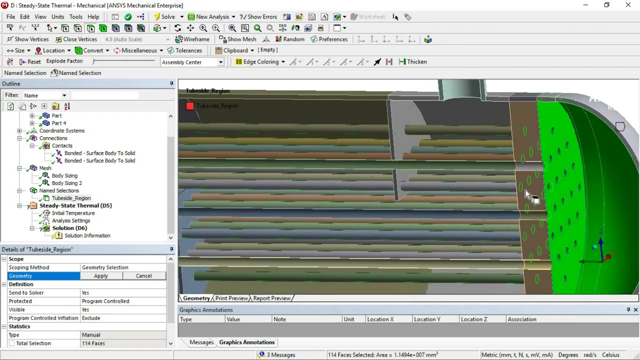 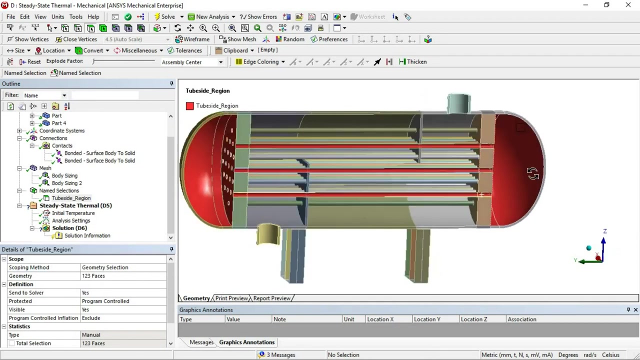 which already created. I will. so these are already created. I will just delete that. and this is what your tube side reason- and here I think we had need to select this- faces also extend to limit. actually, this complete heat exchanger is with a full of this, but here we have taken the 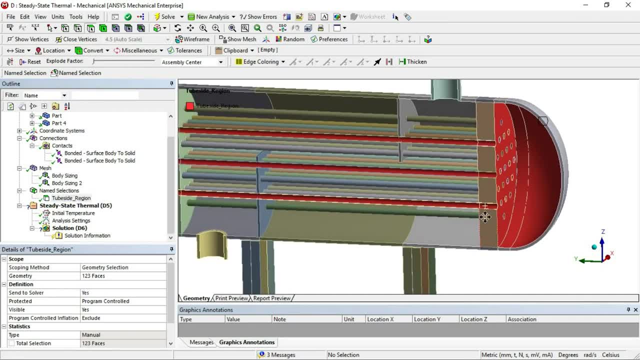 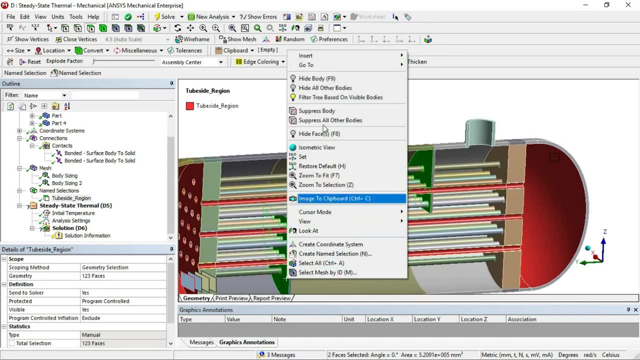 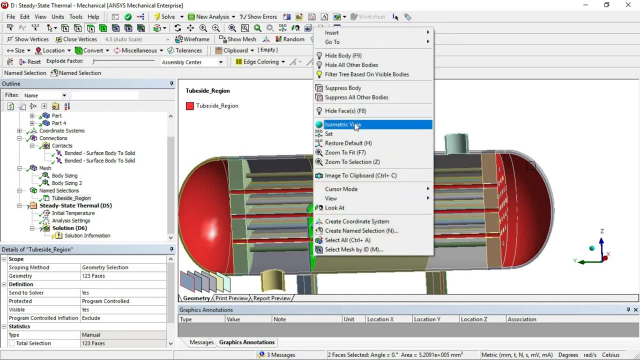 half symmetry. so this is tube side reason and later on we will consider the shell side reason. I will. I will not going to consider this baffles, because I just wanted to tell you what is the effect of this baffle. later on we will see in the next video. there I will going to do the simulation: static, structural. 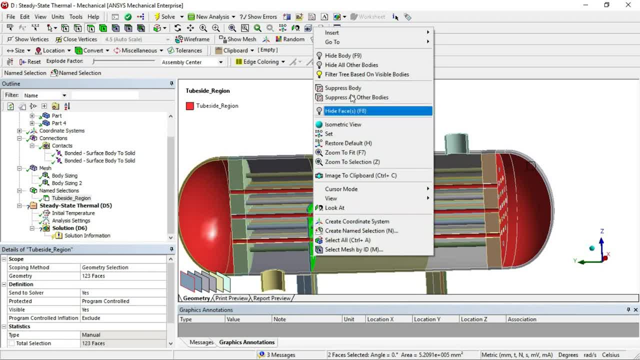 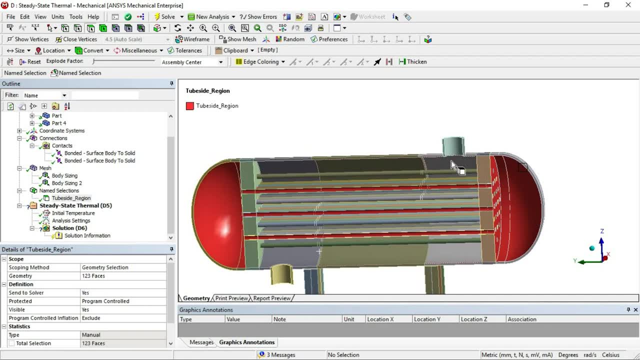 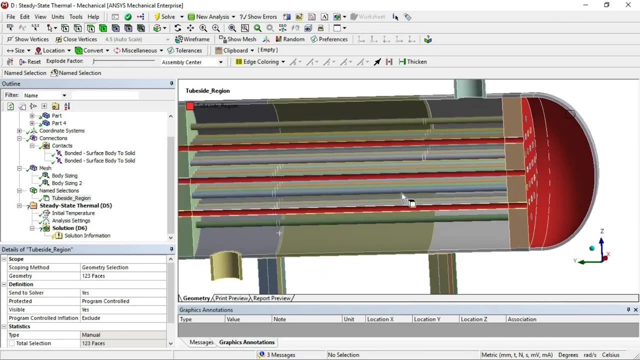 plus thermal. so there you will come to know the difference. the purpose of this baffle: just to create the support for this and also create the flow, what you can say. your Shellside fluid should move like this so that you will get the max surface area. now i will select these tubes. shell side reason: I will do extend. 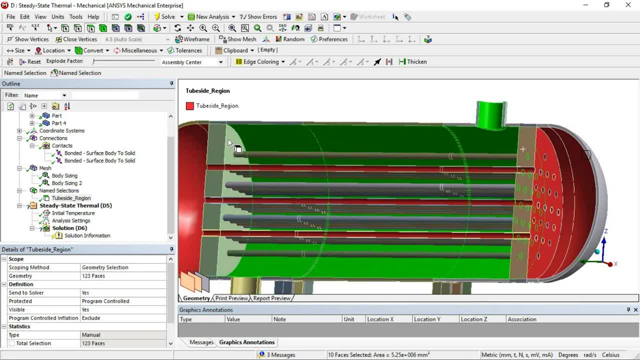 to lim ground. I will select this face, I will select this place and i will also select all the remaining top faces. i will select all the specialty. right now, I don't want to make it tremendously comfortable because this is a hose tube, include a lateral blow which is 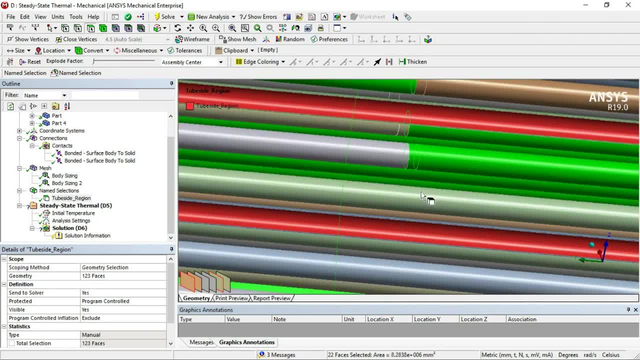 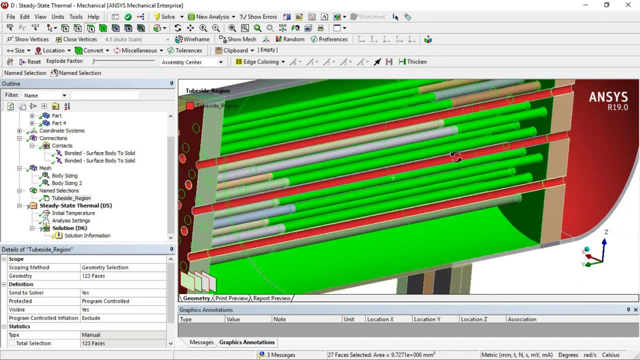 the top stage but the bottom current too. top down on this tube is the top zone of the夫ck. that will help to get it to exclusive area so that the top endactor surfaces outer surface of the mic tubes. here you can use extend to limit option and this 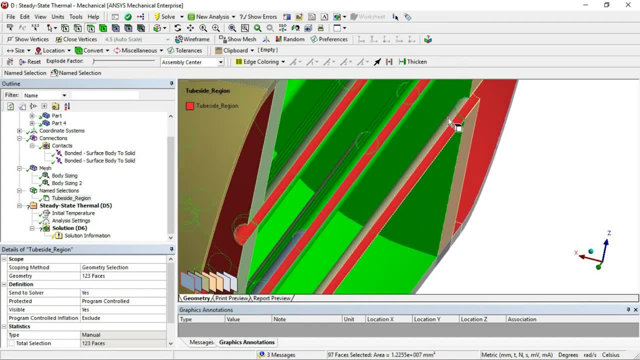 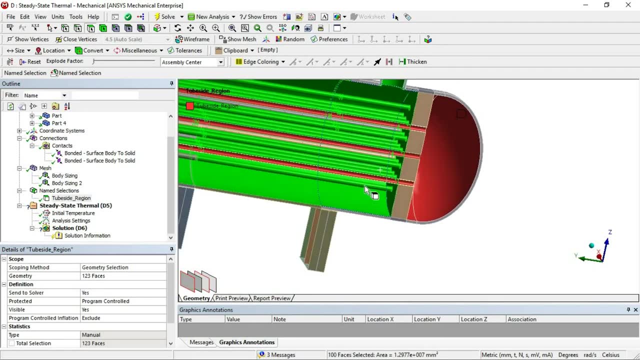 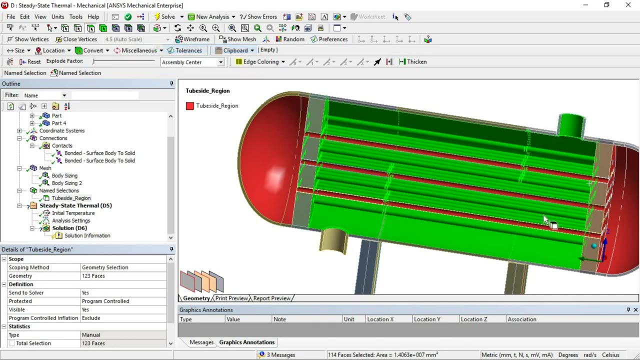 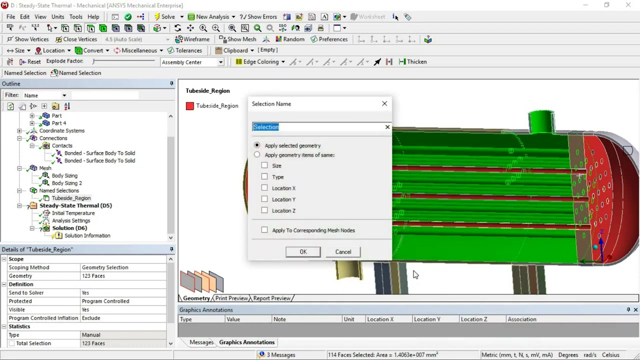 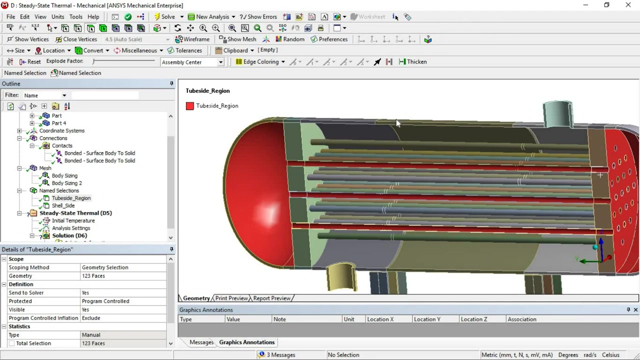 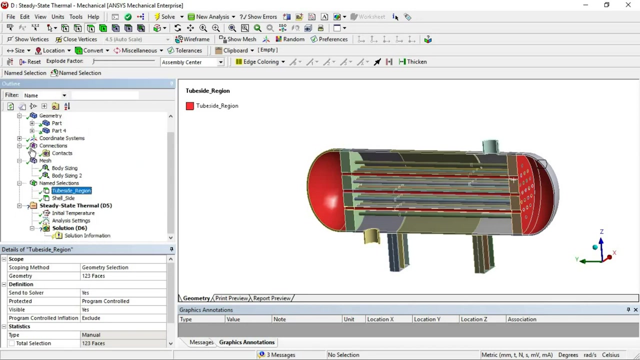 half portion also you can use. there are few tubes are missing still. you just thoroughly cross check: is there any pipe or tubes? are machine extend to limit? I think all tubes are selected. so this is mild shell side reason, because shell side fluid will going to move and this okay. now here we haven't considered the complete vessel, we consider the half symmetry. 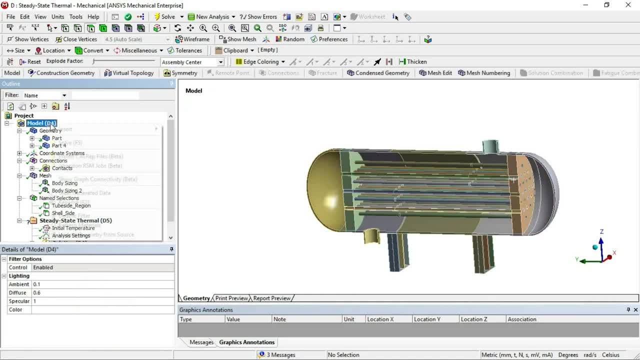 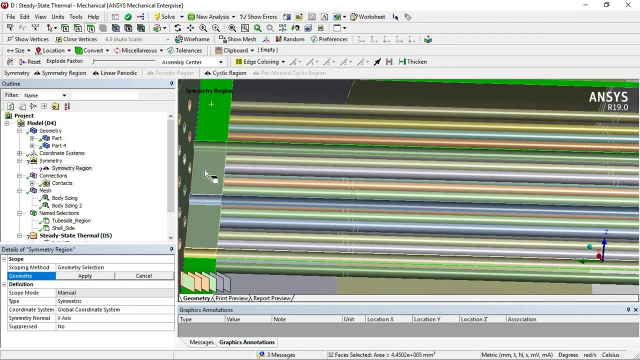 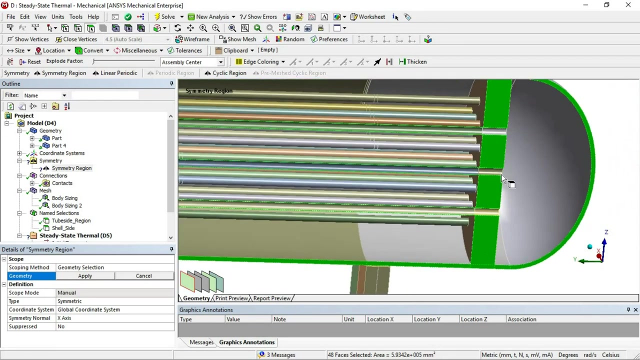 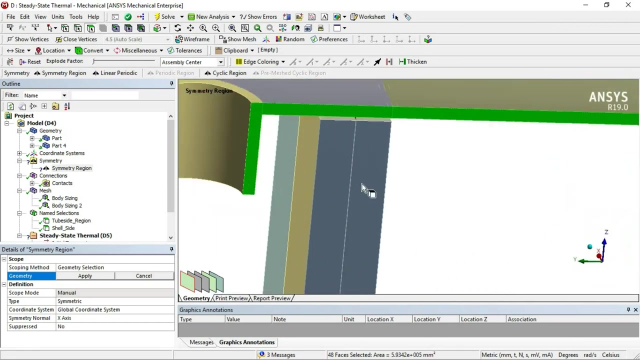 so for that you just go to Symmetry condition, right click inside symmetry andма and here insist symmetry reason. so here you can define the symmetry reason. so I will going to select all these faces on behalf portion you know to select in the symmetry vision, as well as on going to select. 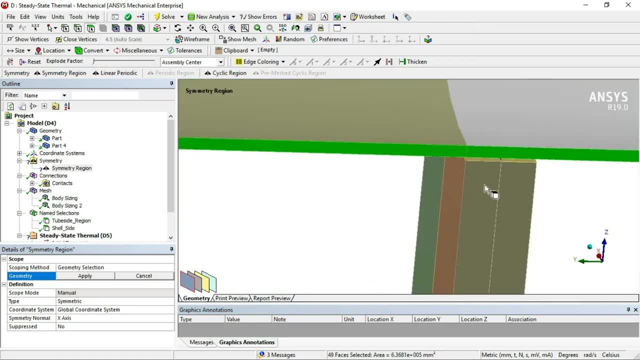 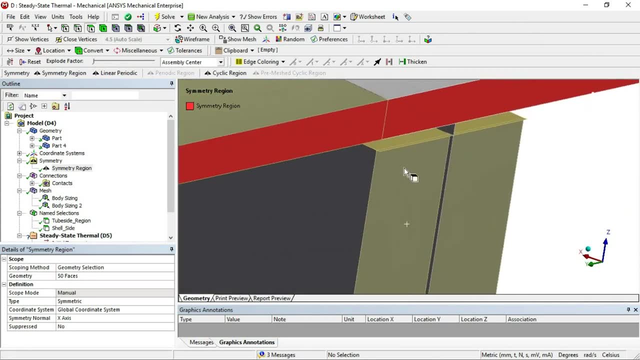 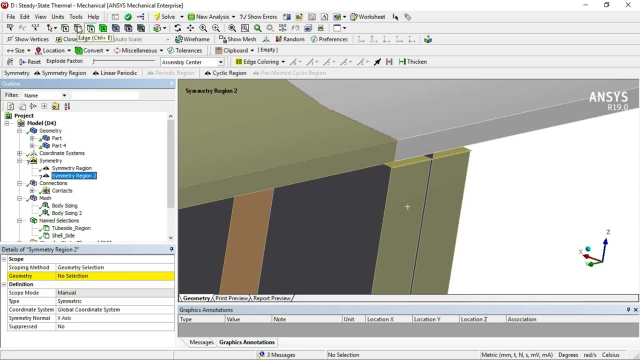 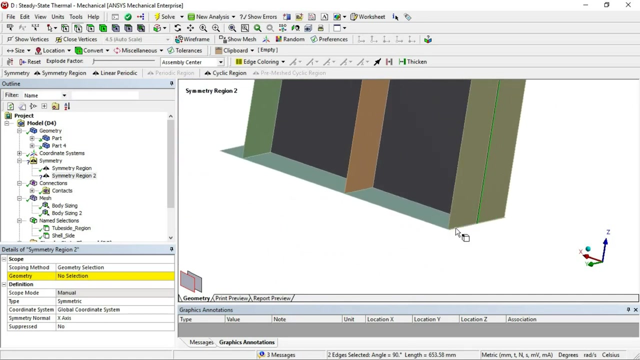 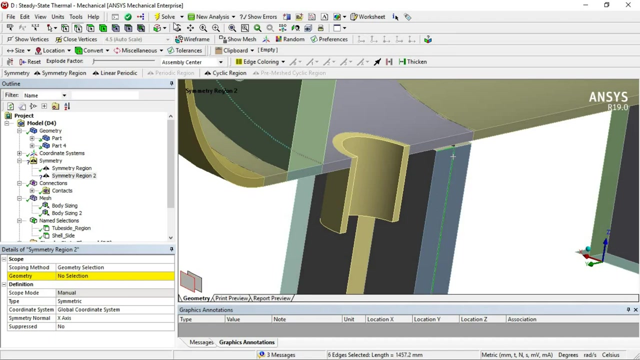 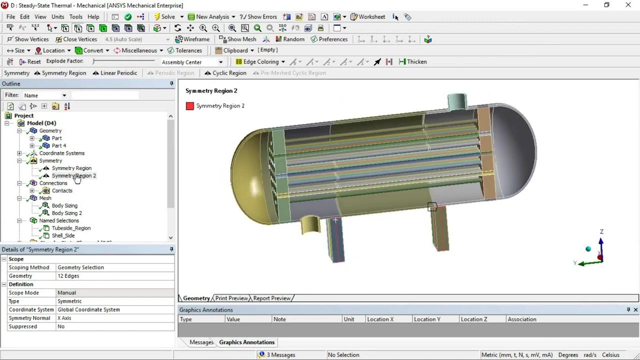 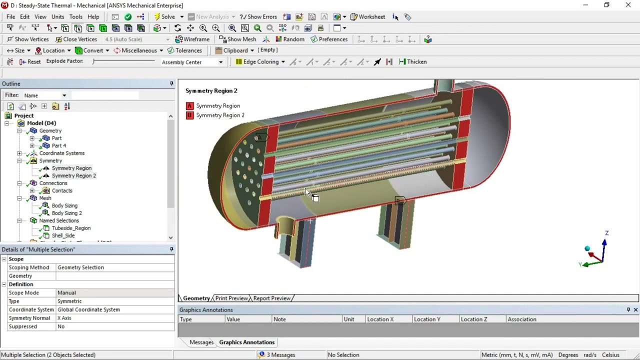 work in design this faces. even I will going to select this edges also insert symmetry region. so there you can define this edges. so I will going to do extend to limit here apply. ok, so here it is done. symmetry is you need to define. just go to model, right click and do this: define your symmetry condition. now our next phase. 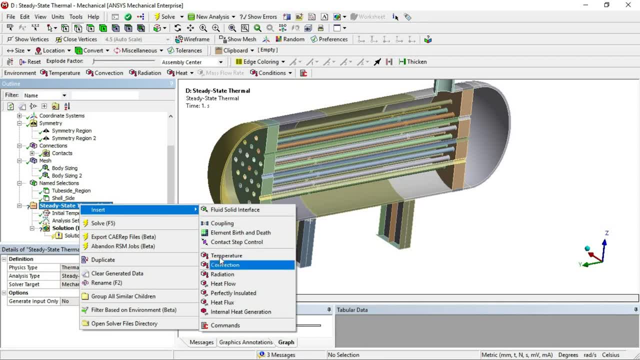 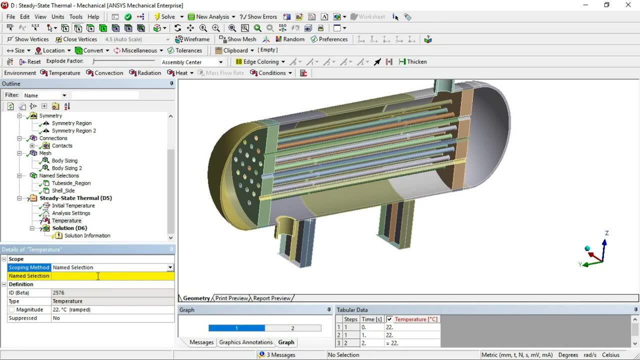 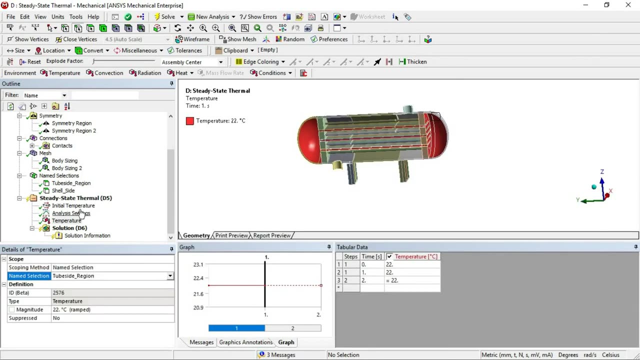 will come your loading condition. so I will going to put the temperature here. I will going to put temperature on a shell side. so here name selection you can tube side first you can define. so there are two loading conditions. so I will going to put here two loading conditions. 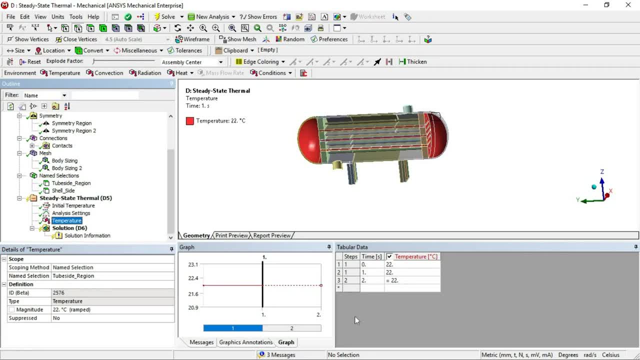 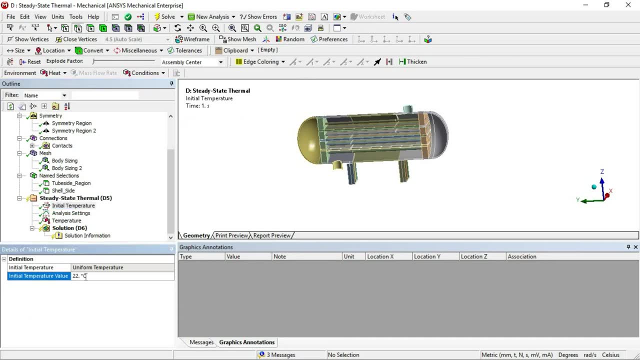 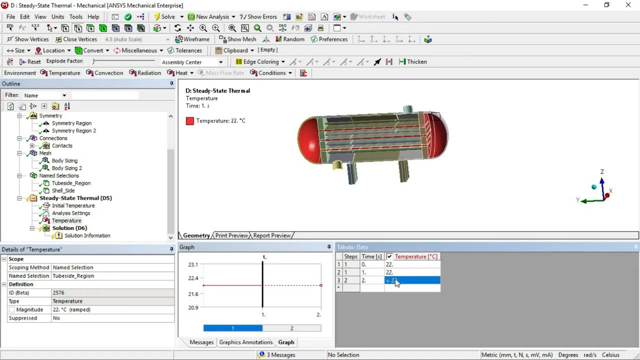 these are already there. and first temperature: we know that first will be here. you can define the atmospheric temperature, that is 22, and the temperature on tube side. first will be first load case, it will be 22 and then later on it will going to increase in second load case. 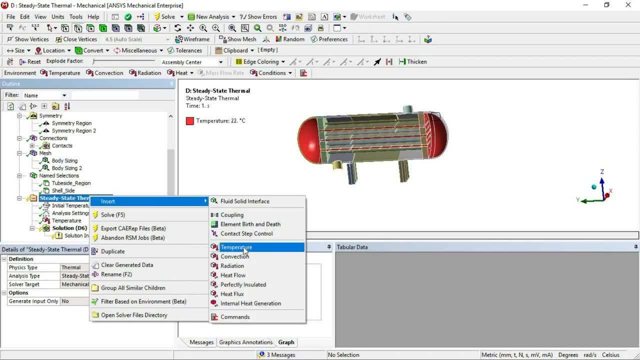 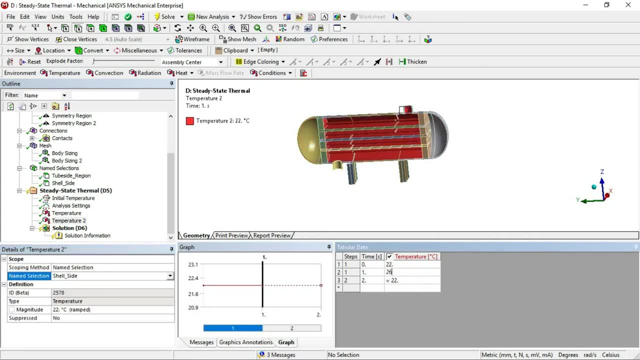 now, similarly, I will going to further in defined temperature. I will keep here on now shell side. so first, ah. so here I will keep 7, here and there I will put here, ah, cell side. now is Carlson's temperature and then later on it will going increase in 2nd load case of 120.. Now, similarly, 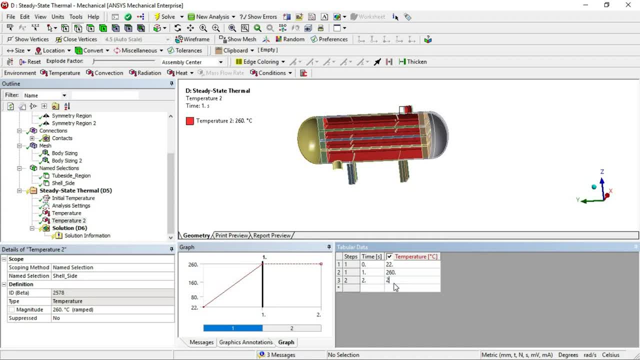 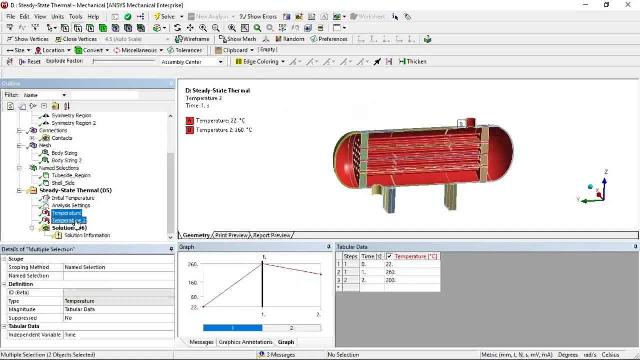 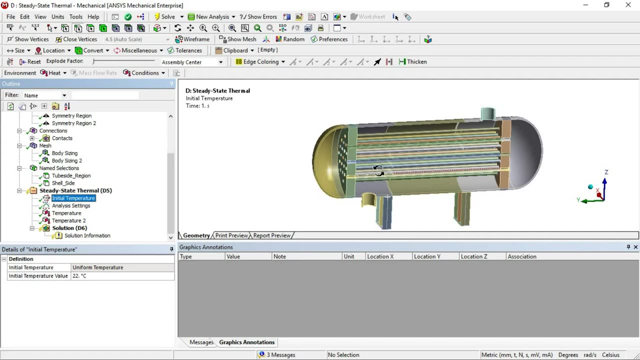 at the start of the cycle and later on it will reduce to 200, so like that, you can define the temperature once it is done. right now, the next loading condition is like it is perfectly insulated, so there will be insulation on the top of this, on the outer surface of this vessel. 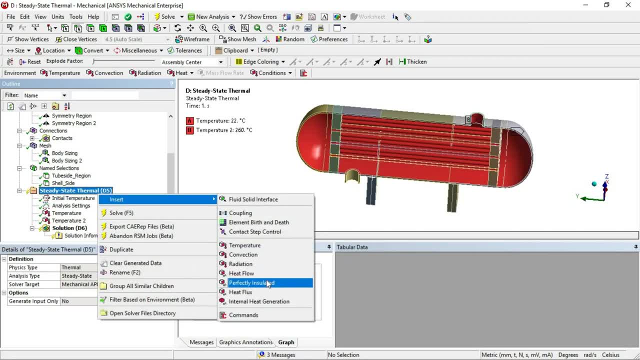 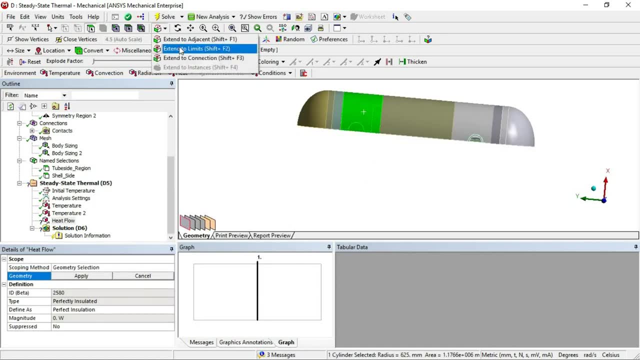 so what i will do? insert here. one option is given that is perfectly insulated, so you can use that option. this is by auto default. you will come to know once you will do this, even you can select this nozzle outer surface says apply. and here one thing will come your in. 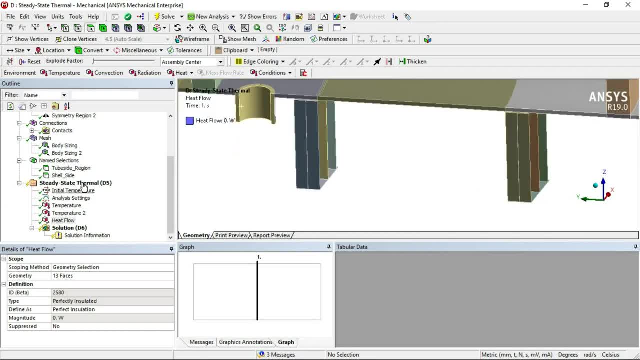 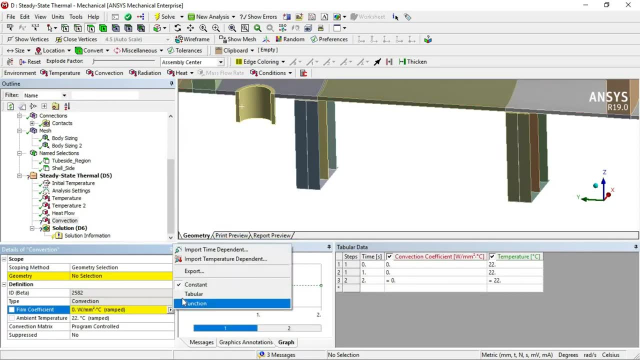 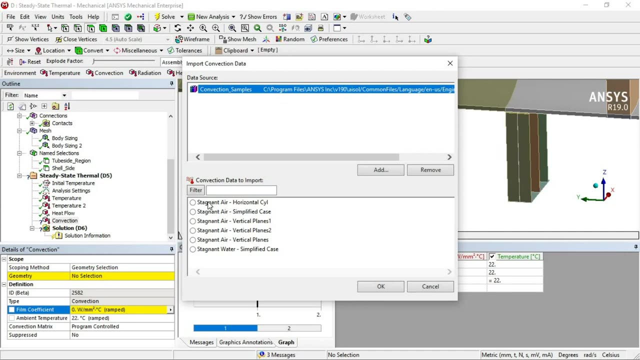 this is some subjected to atmospheric condition. so what i will do, i will define their convection and what i will do here. if you see there are few conditions are defined already in the answers. so like stagnant air, horizontal cylinder, standard air, simplify case, vertical planes. so like that, if you want this. 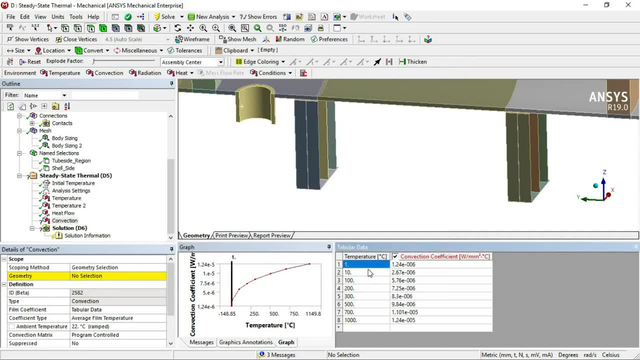 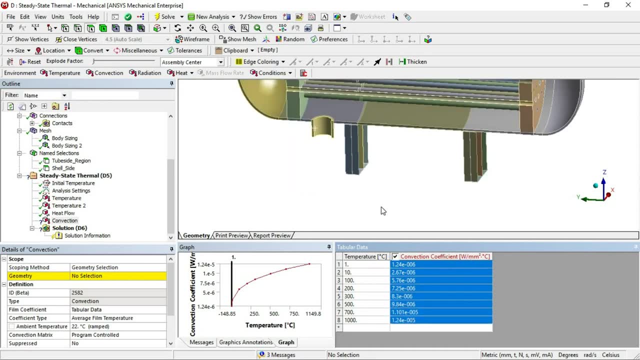 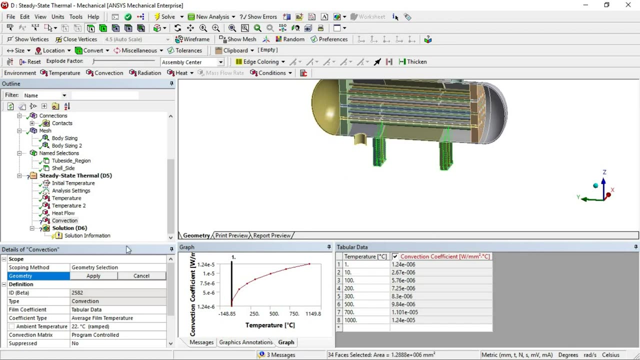 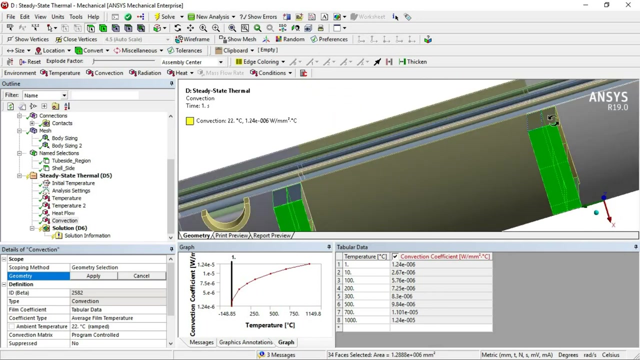 i will pick this by default. it will give us from 1 degree to 1000 degree centigrade, whatever the your watt per meters, mm. squared degree centigrade convection coefficient. so i will select all the conditions apply. right. so here what i am saying: natural convection will going to happen in this. 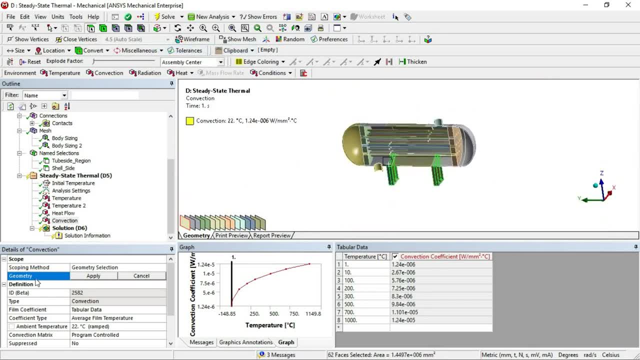 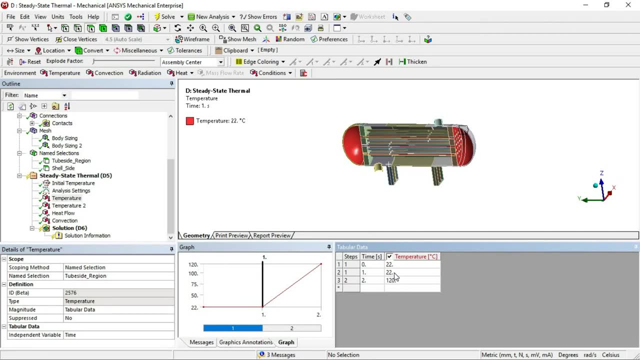 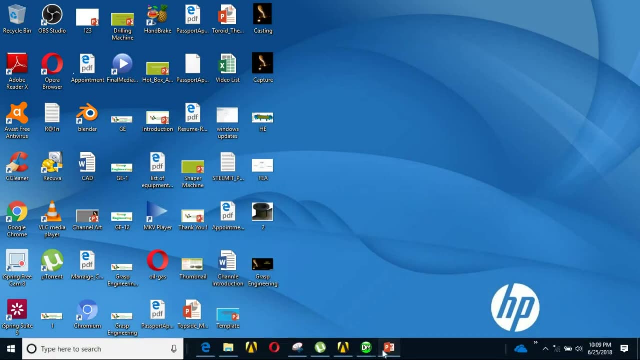 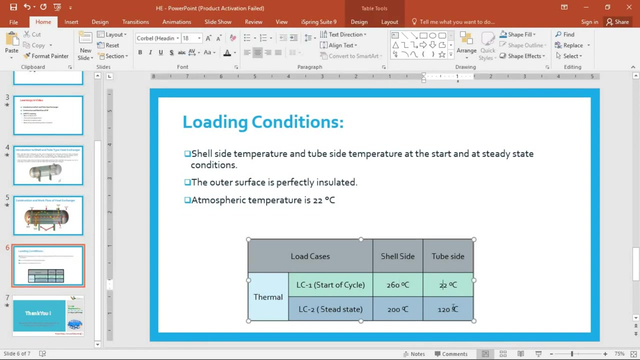 case because that is facing the atmosphere. so this is the condition. so now we had defined the thermal loads. that is a into load condition. if you see, i will show you further our table that we got. the first load case is a 16 komiость, 20 to an average, which is if we tried to 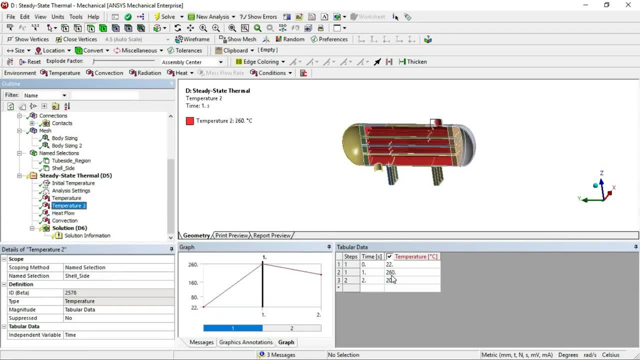 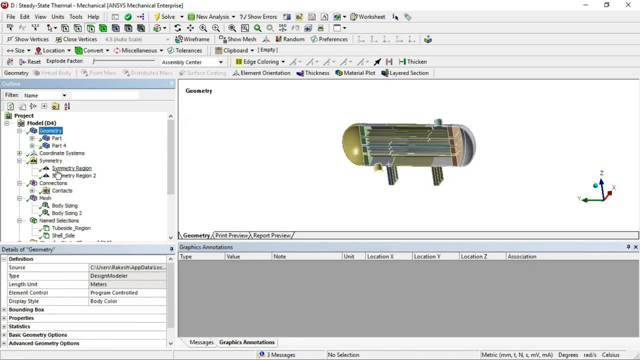 say 300, então dos 922 to 120 K cinnamon stranded method. so we will divide this into official and to囉 mail address: mobile emperor ite emporia asiático are the тут você os cursos? eλλ. article 2 0 dvi. um caso desitus de um dentro da redeção. 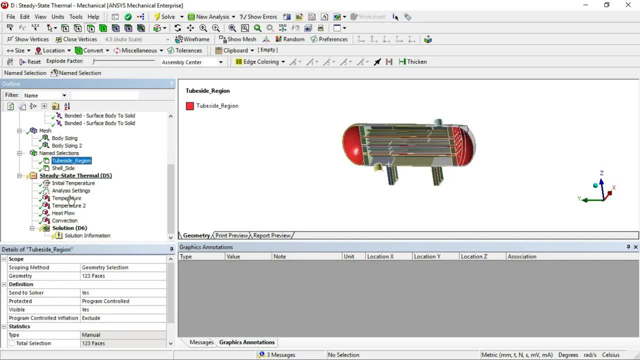 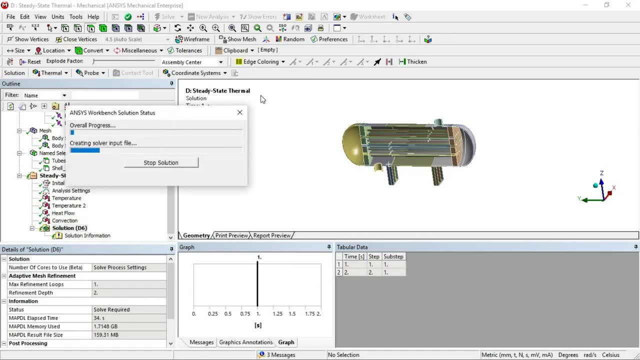 si eupson é uma defesa de também santo valuem a roaming, and so you define what you are sem来 do: condições deрахagem a for the loading set, boundary conditions: okay. once it is done, you just right click and solve. 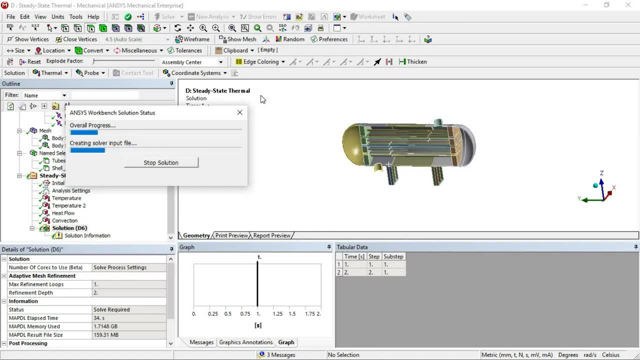 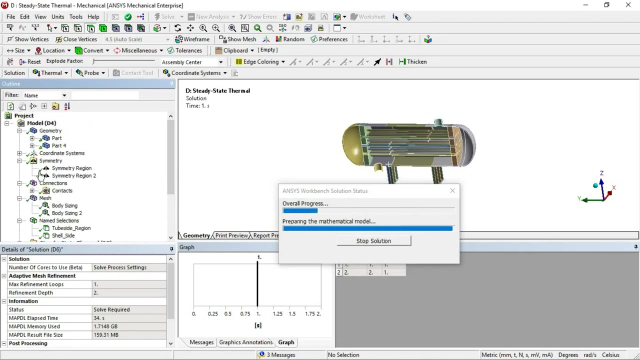 so whatever the loads are there you just define like this, it will take some time. my mesh count is like quite coarser. that's why we are able to solve that within a short period of time. in actual, it will take like half an hour of time, based on your configurations. 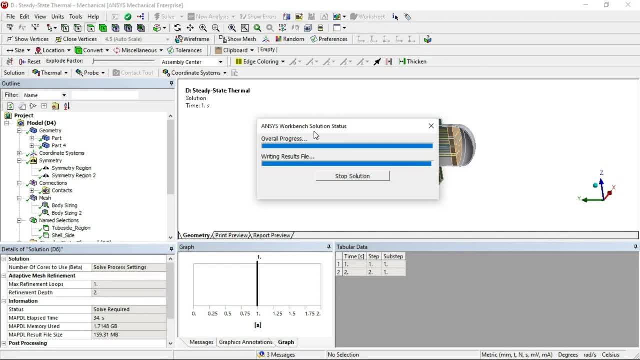 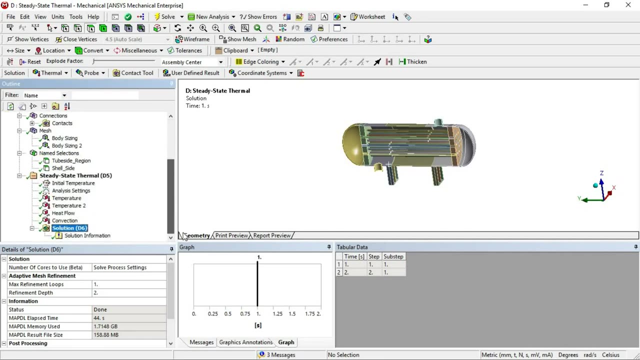 okay, but it is. at least you should take two to three elements across the thickness just to capture the bending behavior. when you will going to do for thermal simulation, there is no need of making concentration, of meshing, but when you will going to do structural simulation, there is a need. okay, now we will. 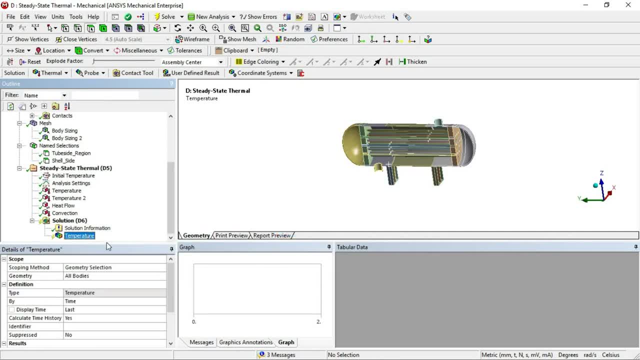 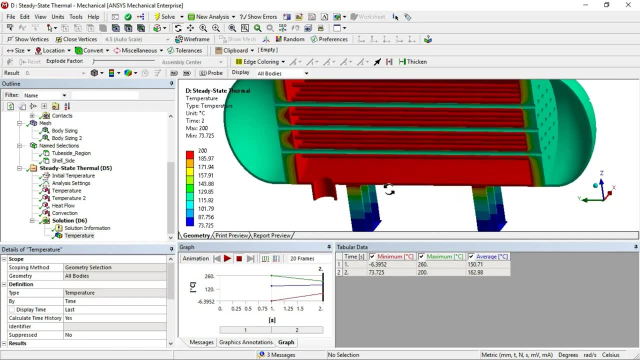 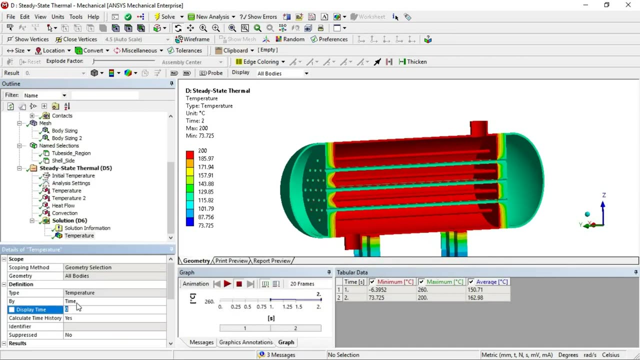 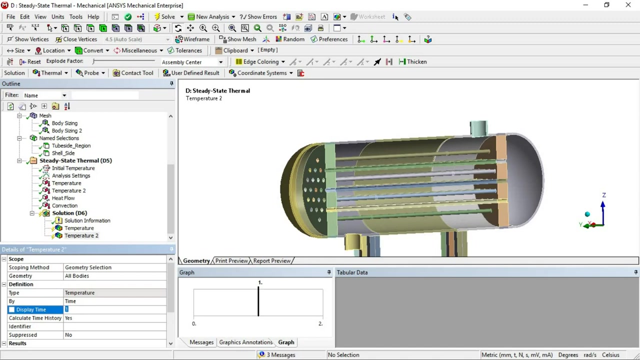 extract the results, evaluate all the results. so if you see, here our thermal results are done and there are like two different load cases, what i will do, i will put display time one for one load case and i will duplicate that and i will put display time second. so we will. 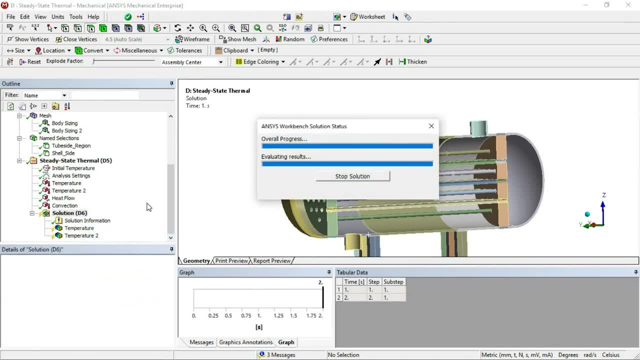 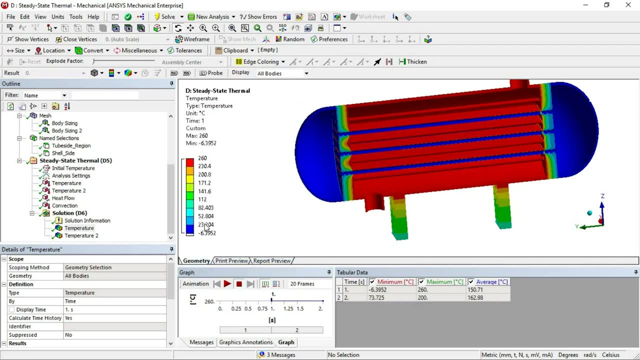 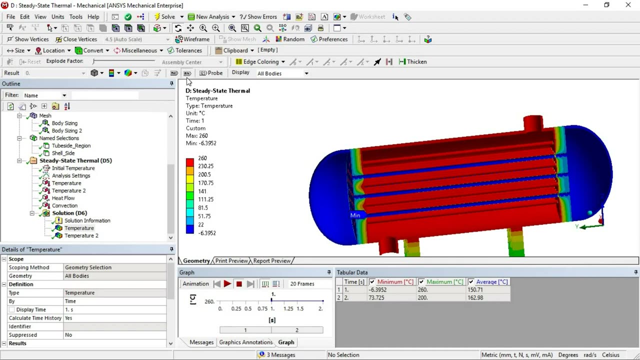 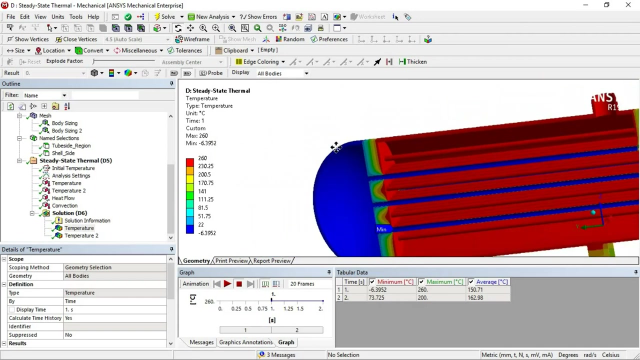 come to know what is the temperature for a load case one and as well as for load case two. so if you see, here for a load case one i am getting the temperature of this is due to contact definition. i will put here twenty two right minimum. it will be like this: so this is at this which is localized. 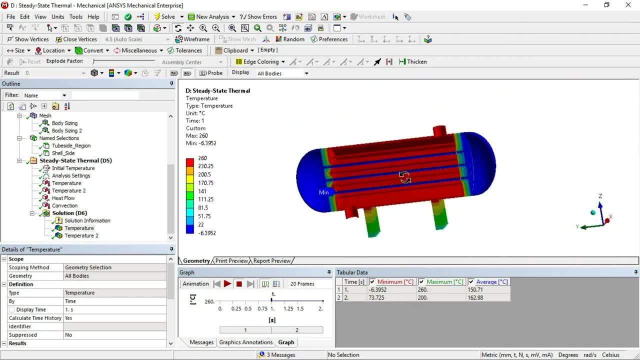 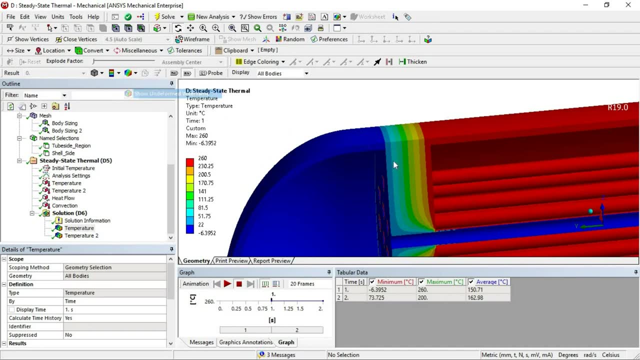 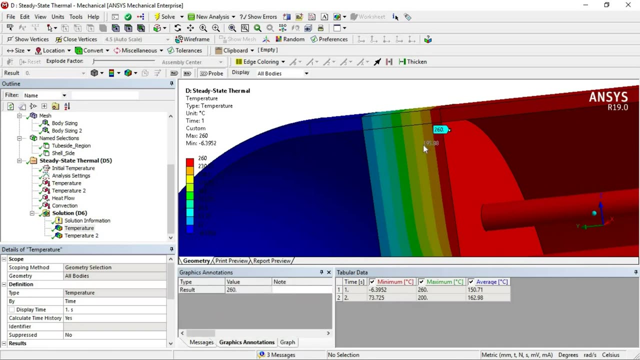 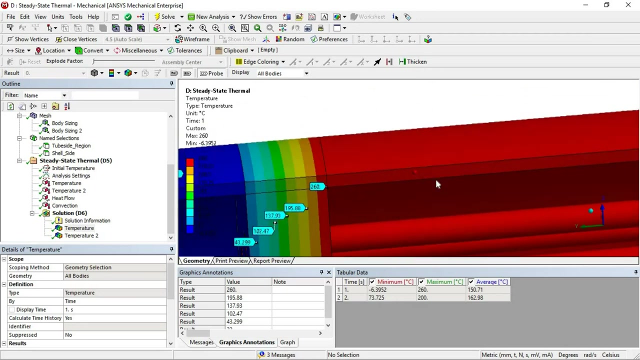 and maximum it will be two sixty. so what we will see, we will see that reason. i will display this reason right and here. if you probe, you will come to know. it is two sixty here and gradually it is reducing. you can see. see, here it is 22. so like that we will get the gradient across this. even this is perfectly. 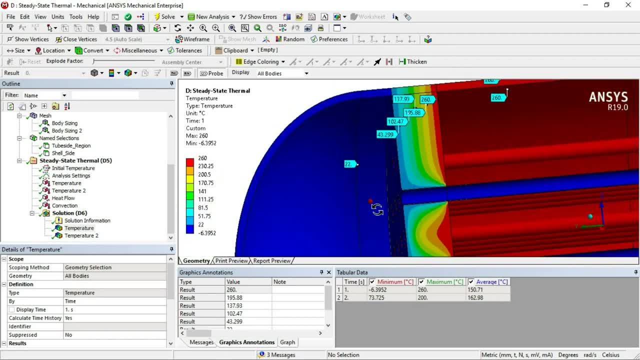 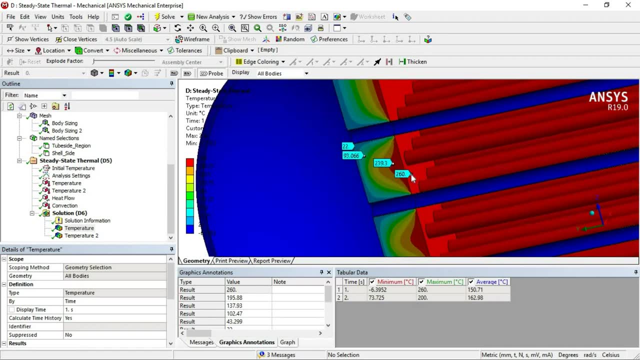 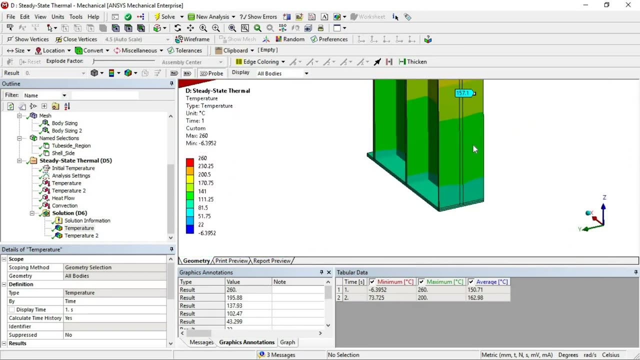 insulated, so that's why there is no temperature loss. but here it is: your tube side is at 22 degree centigrade and your shell side is at 260 degree centigrade. okay, similarly, here also you can see the temperature gradient. it is like from atmospheric. this is we had. 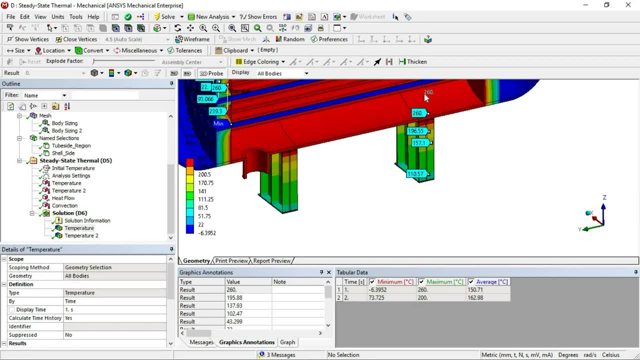 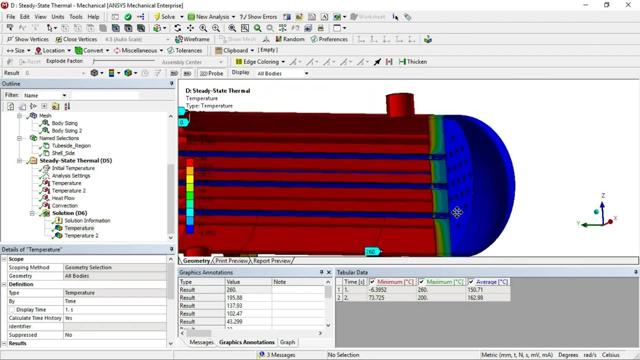 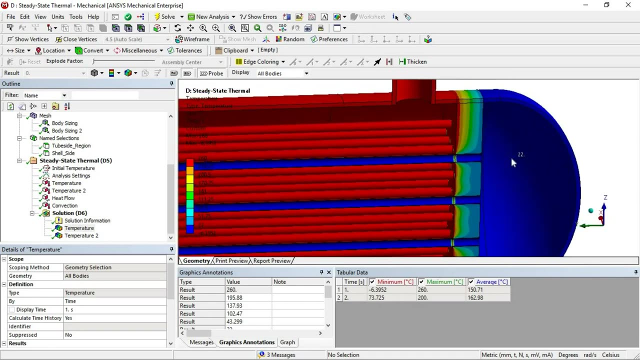 kept it at the atmospheric. so the due to the conduction, you will find the temperature is reducing up to 110 degree centigrade. so if you have, you know testing results or you can say actual field results which you had measured for using thermocouple, so you can also apply. 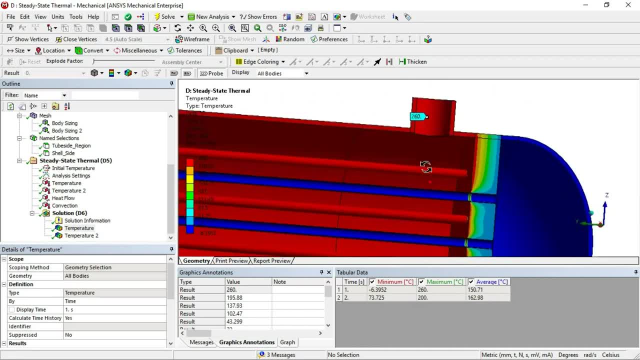 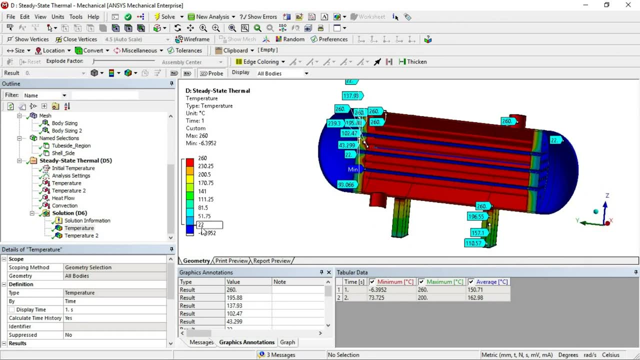 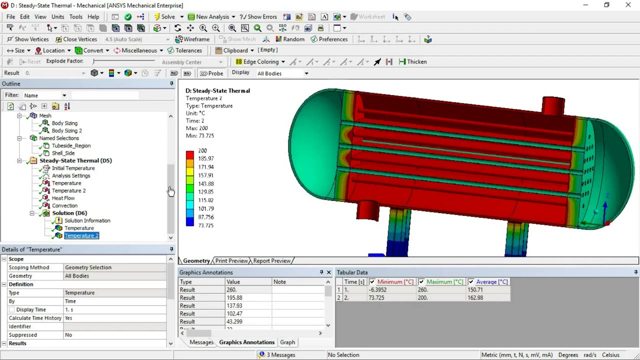 like that. like that, this is the worst case scenario, right? so this is the the temperature output for load case one, where we had applied from 22 atmospheric to 260 degree centigrade, and the same we are getting, and similarly for load case two: right load. 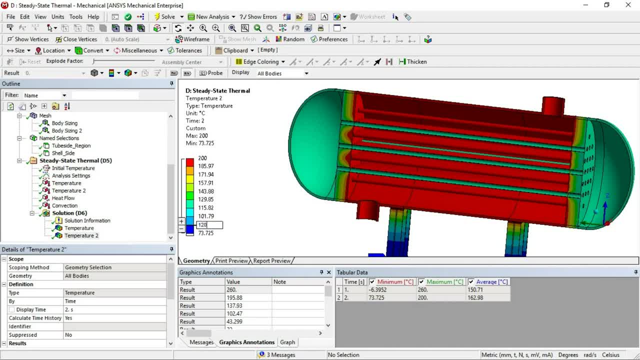 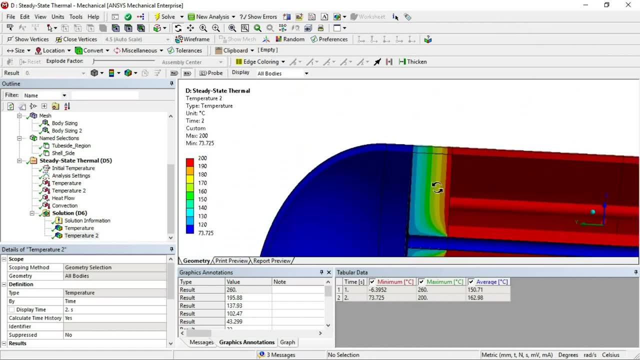 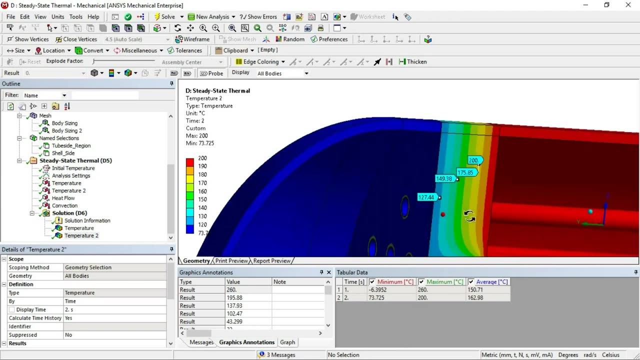 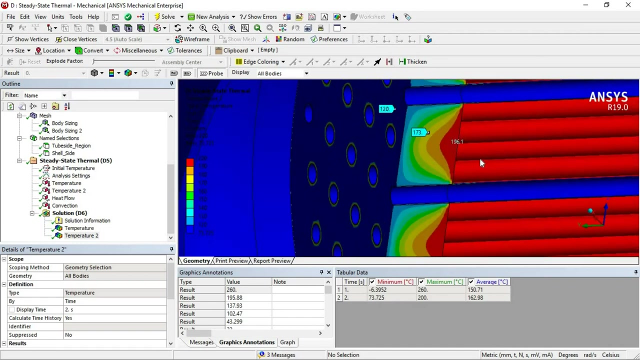 case two: we are getting from 120 to 200 and similarly we are getting here also gradient. so we will check that further. here it is 200 right, so 200 to 120. you can see here. here also we will further cross check. it is like to so shell. 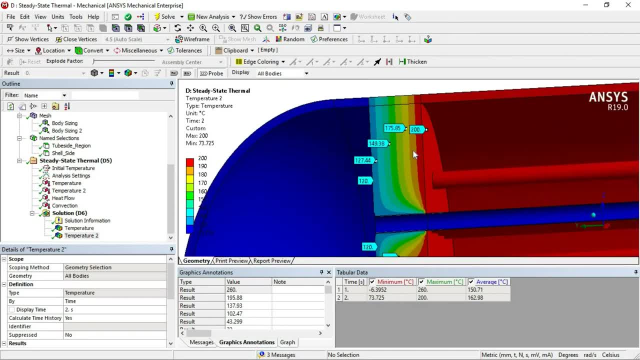 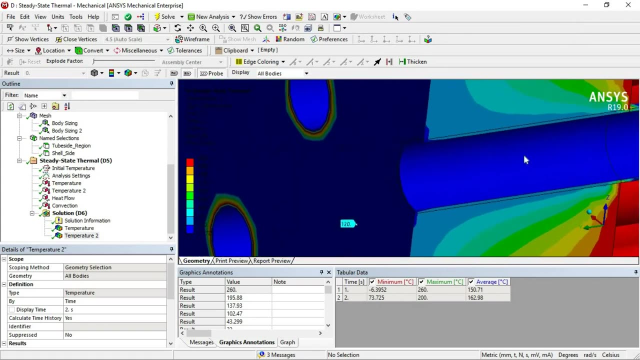 side to tube side. here if you see, the temperature gradient is less in this case compared to earlier. in earlier case it is like from 260 to our atmospheric temperature that is 22. so here it is less and you can see here inside the tubes also as we tube side fluid here. 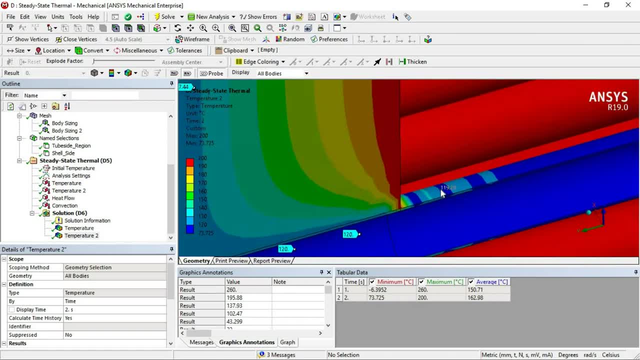 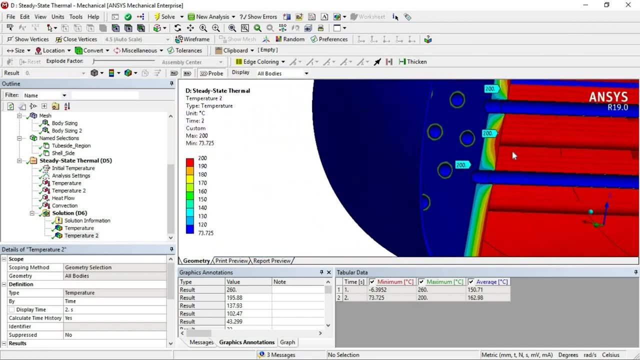 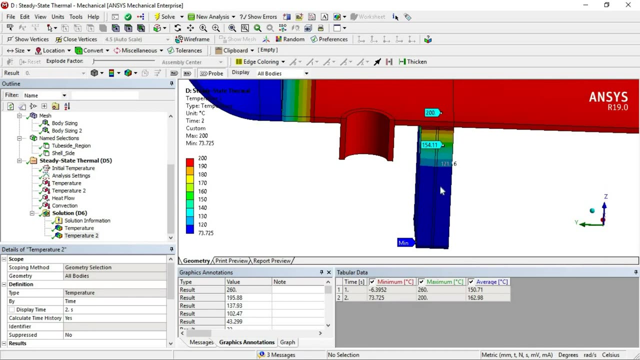 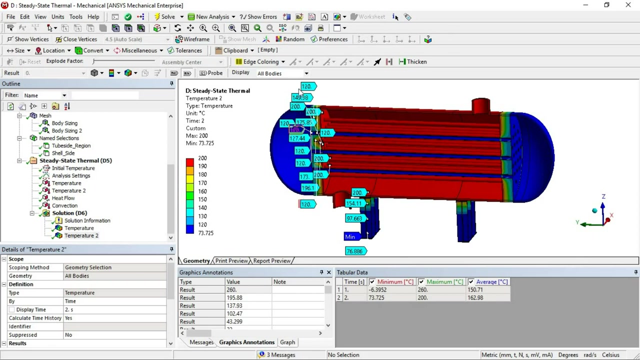 it is 120, but here, if you see outside this tube, it is 200. inside the tube you will find 120, okay, and here also you can see the gradient 200 to 76, okay. so like that we need to do the thermal simulations if you have proper results or if your temperature results low. 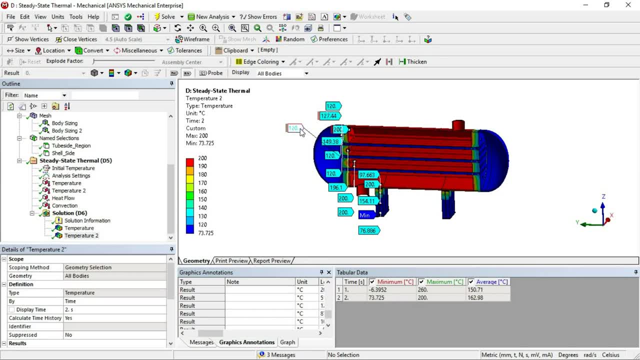 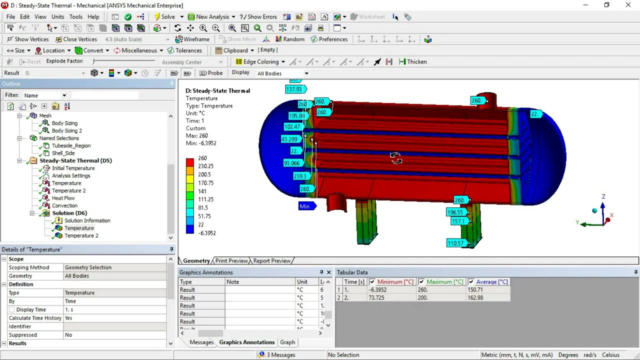 measurement which you had done at your field. then, based from the thermocouples, you can apply that respect to temperature at your different tube and shell side and you can do the thermal simulations. okay, so that's it like that. you can do thermal simulation for different configurations of. 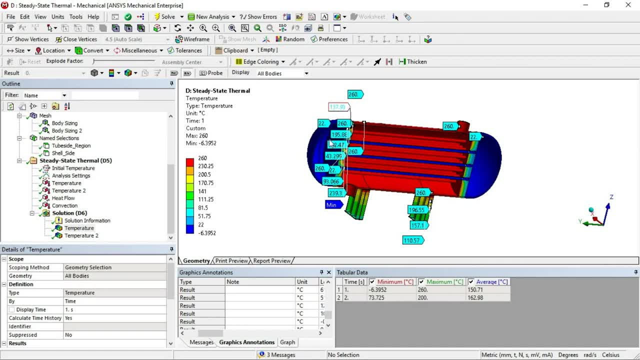 pressure vessels as well as your heat exchangers. I will continue this video in next. there we will see what are the results, or you can say what are the thermal stresses for this- to configuration at the start of the cycle and at the end of the cycle. if I will continue now, then you will find that 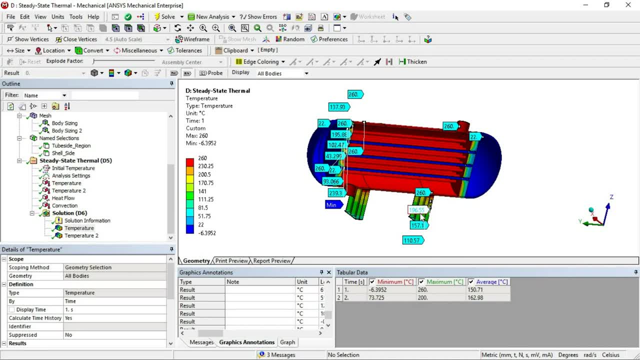 there will be huge time already it is like half an hour- but what I will do, I will split into two parts. first part will be your thermal simulation and second part will be static simulations. okay, guys, so thank you. thank you for your time and keeping patient for watching this complete video.